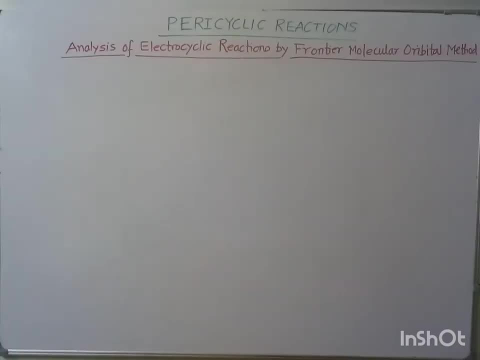 Hello students, welcome you all. Now, in my today's lecture I will explain you the analysis of electrocyclic reactions by frontier molecular orbital method, that is, by FMO method. So in my last lectures I analyzed the. I have explained the analysis of electrocyclic reaction by 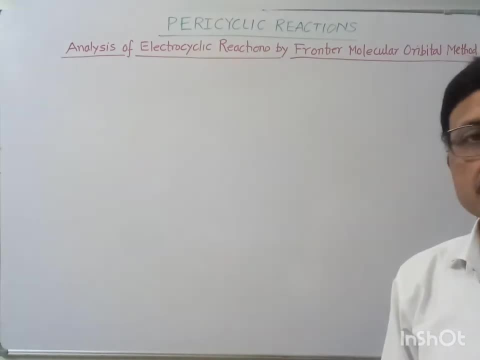 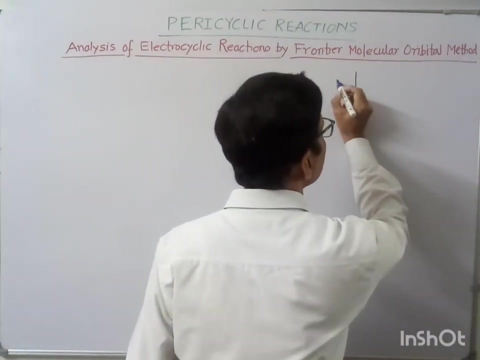 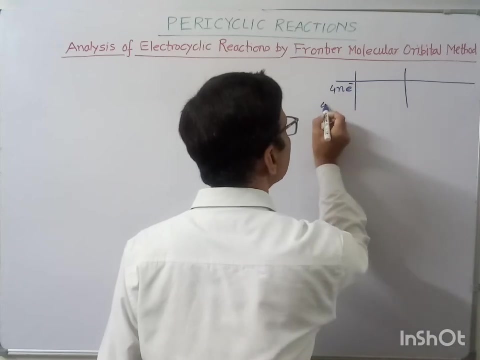 orbital symmetry correlation method, that is, by using the correlation diagram. So here I will explain this electrocyclic rule with the help of FMO method. So already I have explained the electrocyclic selection rule. So for 4n electron system and for 4n plus. 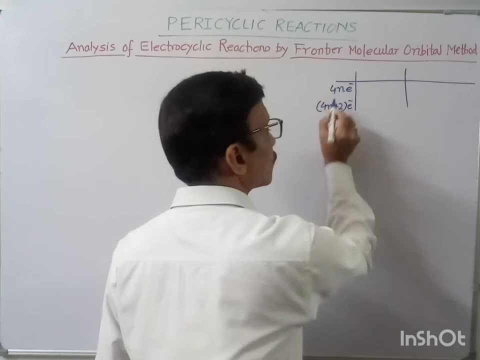 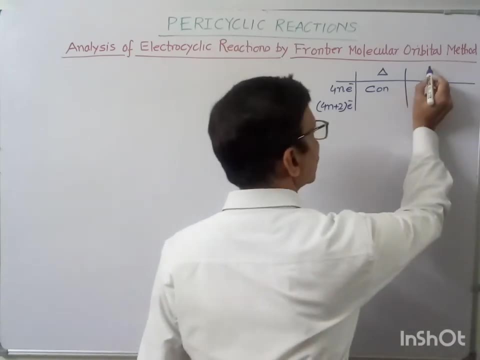 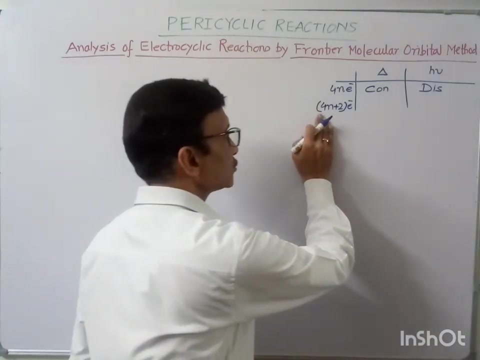 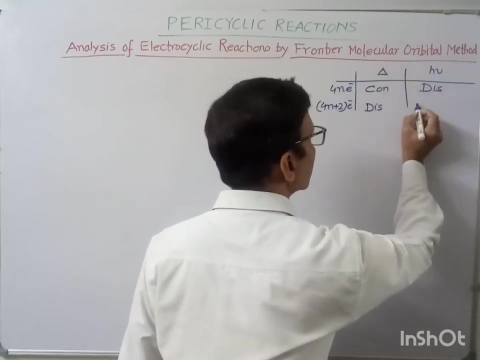 2 electron system. So for 4n electron system, under thermal condition common rotation of molecular orbital occur, whereas under photochemical condition this rotation of molecular orbital takes place For 4n plus 2 electron system under thermal condition this rotation of molecular orbital takes place Under photochemical. 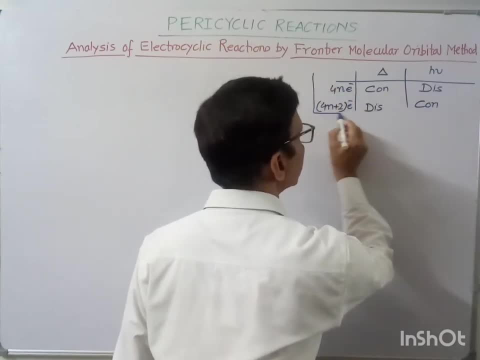 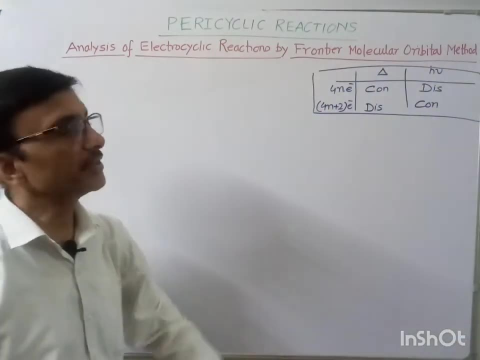 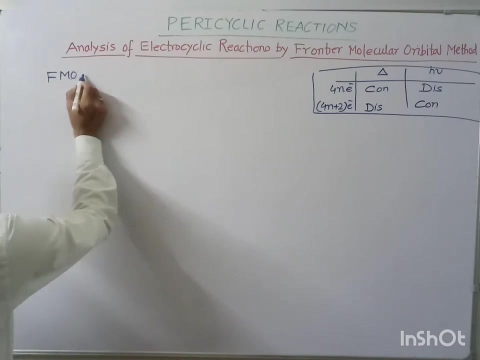 condition, common rotation of molecular orbital takes place. So this is the selection rule that we have to analyze with the help of FMO method. So we know that frontier molecular orbital, FMO, two frontier molecular orbitals are there. One is called as the MOMO, that is, highest occupied molecular orbital, and another is 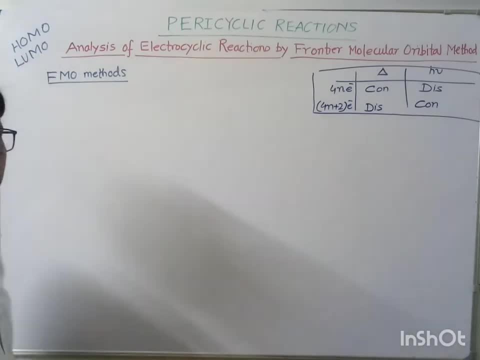 called as the LUMO. MOMO and LUMO is involved in any reaction, So lowest unoccupied molecular orbital. So these are called as FMO and LUMO In the LUMO. are you aware of SOMO recently we are? 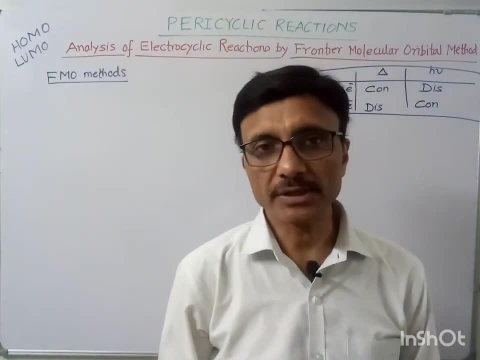 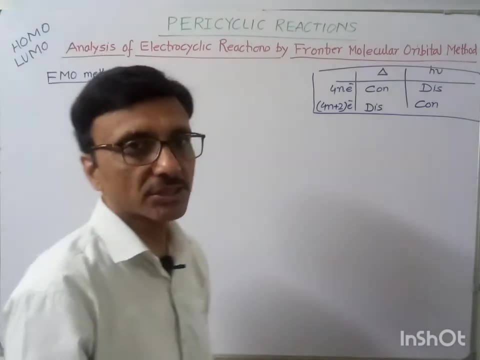 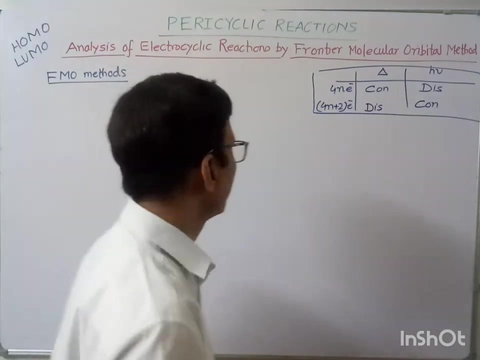 talking about this. it is a very important group Here. in this lecture I will explain as the two frontier molecular orbitals now, so in this method. so as all of you know this, electrocyclic reactions, either it may be ring closing reaction or it may be ring opening reaction. so when we analyze the ring closing reaction, so two. 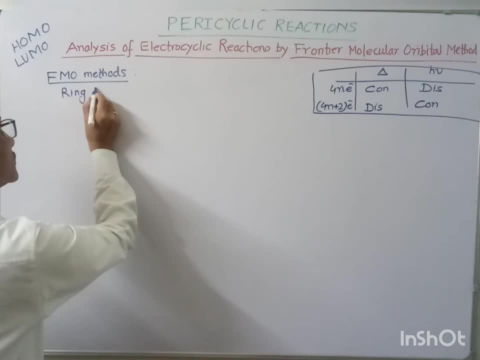 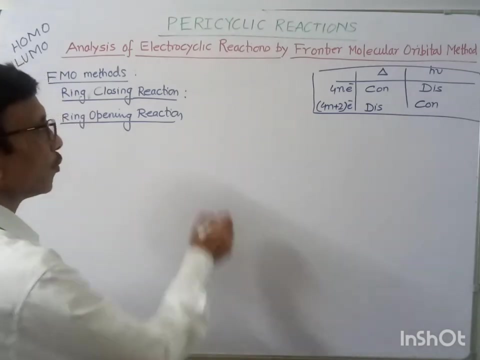 type of reactions we discuss in electrocyclic reaction. one is called as the ring closing reaction and another is the ring opening reaction. ring opening reaction: two type of reaction we discuss. so in ring closing reaction, in ring closing reaction, in FMO method. FOMO is involved. 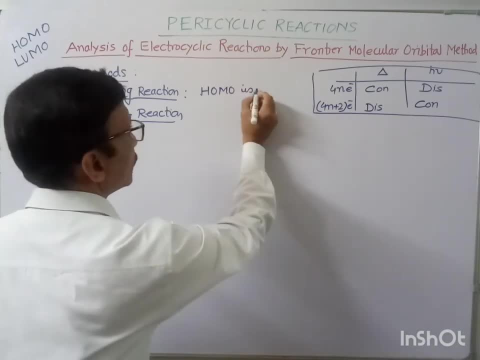 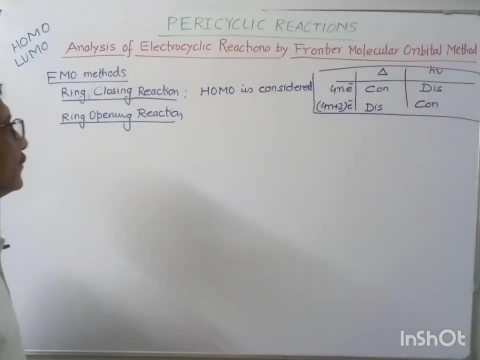 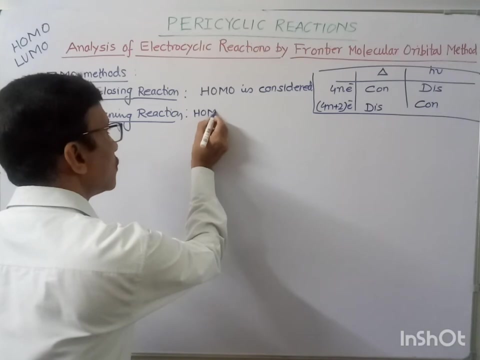 FOMO is considered, or we can say: FOMO is considered during the analysis, whereas in ring opening reaction I will consider FOMO and LUMO. so FOMO and LUMO is considered so usually. otherwise we can also consider the FOMO only, but here the FOMO is considered only, but here the LUMO is considered only, but here the FOMO is considered only and here the T assimilior reaction is considered. returning the loan of LUMO to FOMO and LUMO: tomorrow on I will discuss FOMO for consideration of the crack reaction中 sliding reaction, I' manière dalla dietera vedetah. 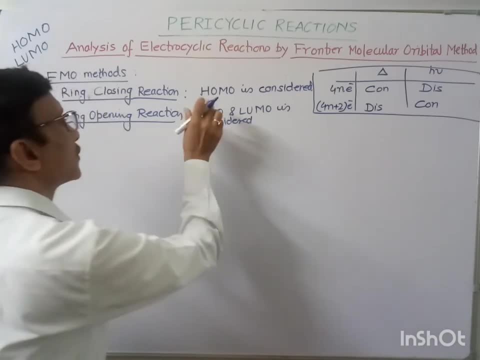 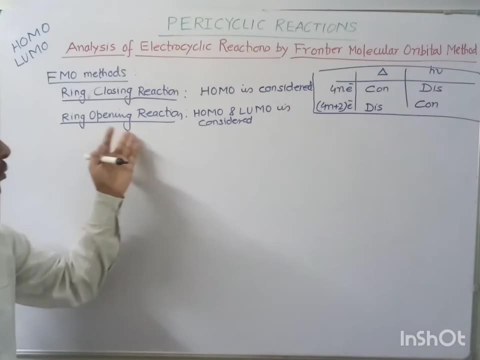 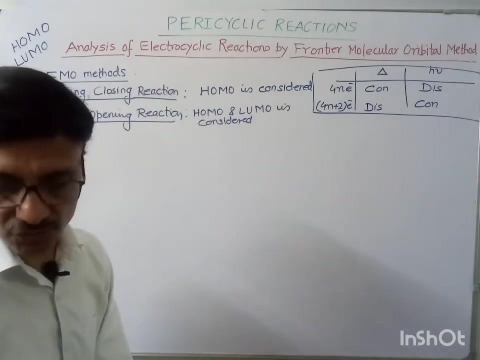 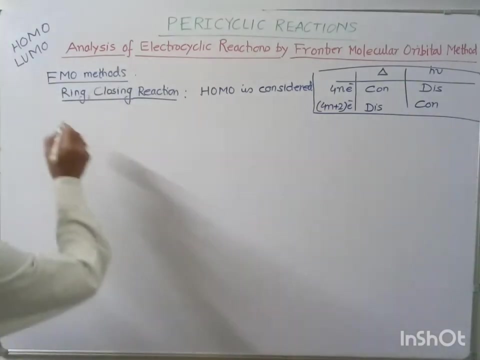 usually. otherwise we can also consider the FOMOesa, but here I will consider HOMO as well as HUMO or ring opening reaction. okay, now let's first see the ring closing reaction. so first of all I will discuss the ring closing reaction. so, as I told, two type of system we usually take in. 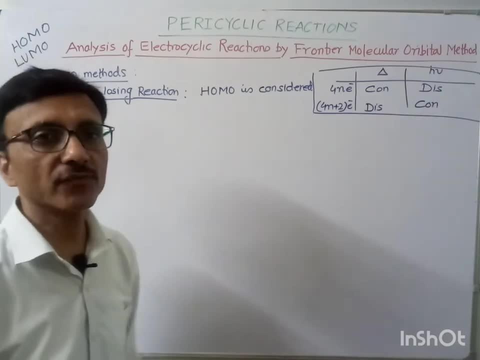 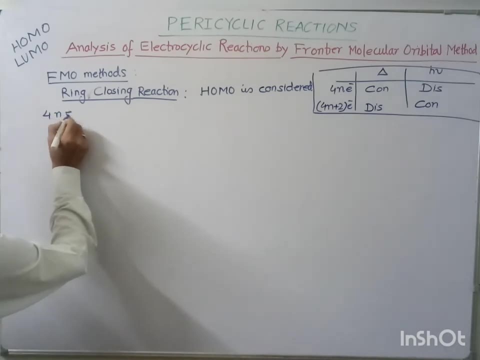 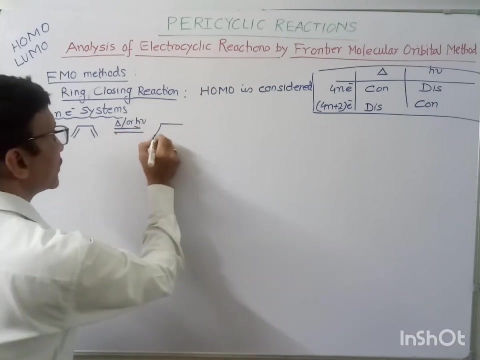 pericyclic reaction: 4n electron system and 4n plus 2 electron system. so if I take 4n electron system, okay, for example, if I take, suppose, this butadiene, this impedance of heat or impedance of light, that would be converted into 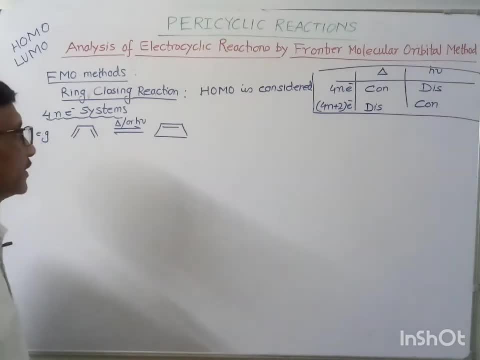 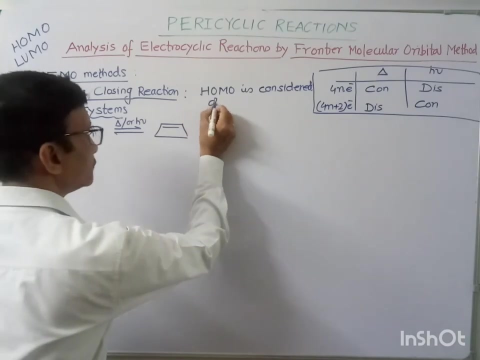 cyclic building that would be converted into cyclic building now. so in this reaction- so this is ring closing reaction, this is the ring closing reaction. okay, so what I have told, in ring closing reaction we take the HOMO of reactant. HOMO of reactant is taken. so in this case, the, this is deutlich. and for the ter, hmm, which contains carta, theology, is shown. falta volta electricity is written. 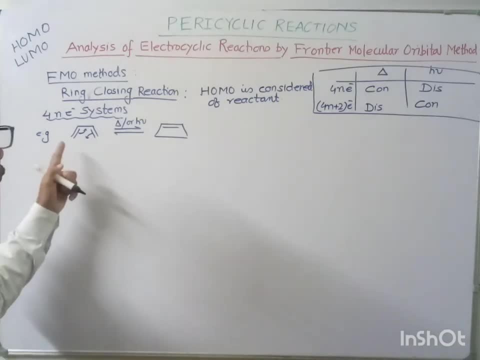 is the four molecular orbital. Four molecular orbital: psi 1, psi 2, psi 3, psi 4.. So four molecular orbitals are there. So for example, this is psi 1, psi 2, psi 3, psi 4, like this: 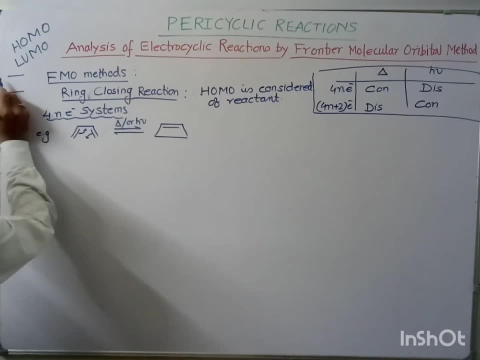 So pi 1, pi 2, pi 3, pi 4.. How many electrons are involved in this butadiene? Four electrons are involved. Four pi electrons are involved during the reaction. So these four pi electrons can be filled in this molecular orbital. So first of all we fill two electron in first. 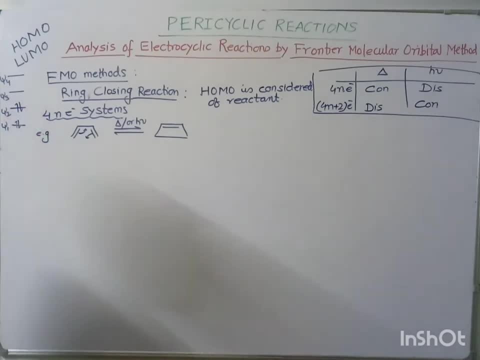 molecular orbital, then next two electron in second molecular orbital, So this is psi 2.. So psi 2 is called as the HOMO, Whereas this is called as the NU HOMO. So what should I take? We take the HOMO of the reactant molecular orbital. So if we take the HOMO is psi 2.. 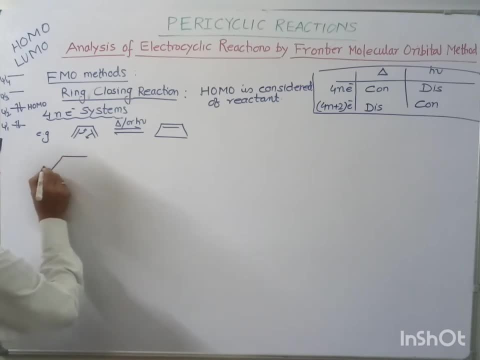 Psi 2 of this reactant, Psi 2 of butadiene, we can write: We can write the psi 2 of butadiene as this: So this is what is: psi 2 of butadiene. Psi 2 of butadiene is plus, plus, minus, minus. This is plus, plus. 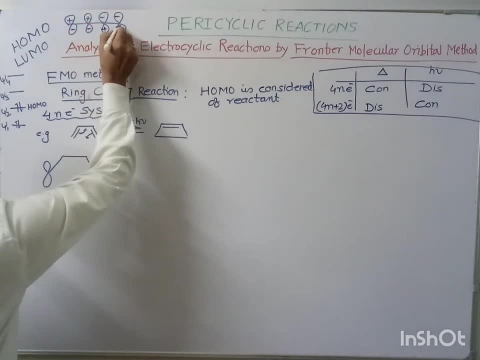 minus minus. So this is the psi 2 of butadiene. In psi 2, how many nodes are present? One node is present and that one node- it passes through the center. So this is psi 2.. So 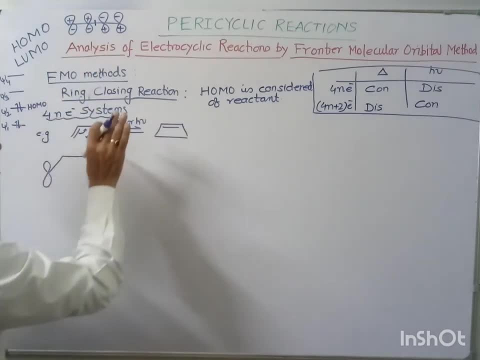 this is psi 2, and here, during this analysis, we are only concerned with the end molecular orbital, This one and this one. We are not concerned with this middle molecular orbital, We are only concerned with the end molecular orbital. So that would be sufficient to analyze. 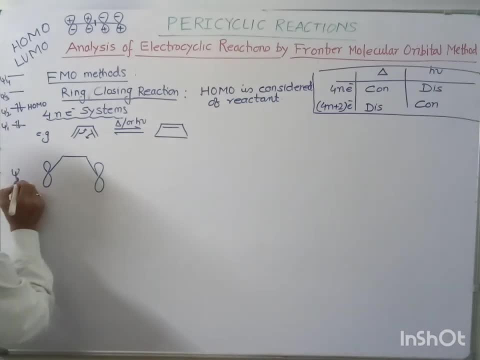 such reaction. So this is psi 2 and this psi 2 is the even molecular orbital and even molecular orbital. what I told, The end orbital has the opposite sign, plus and minus, because this is even molecular orbital. In the same way, psi 4 is also even molecular orbital. So the end orbital that would have 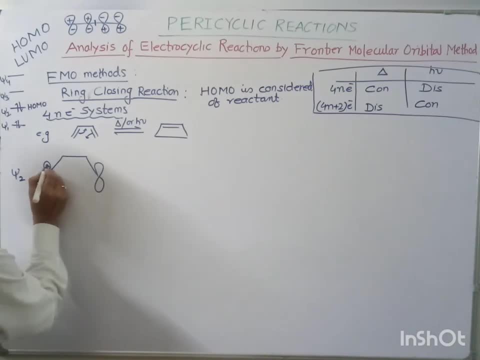 the opposite sign. So this will have the plus sign, this will have the minus sign, this minus, this plus. So this is psi 2.. Now what we can do here. So either under thermal conditions, So just this psi 2 is, psi 2 is the HOMO- under thermal conditions. First of all, I 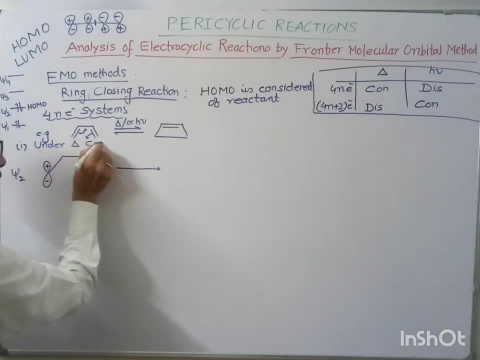 should write here: under thermal condition. So we are discussing this reaction under thermal condition. under thermal condition And under thermal condition, only psi 2 would be the HOMO. Okay, So this is under thermal condition, and whether in thermal conditions? 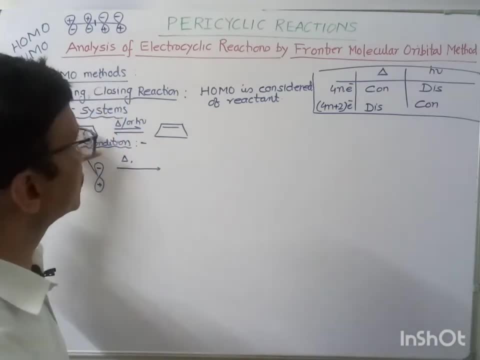 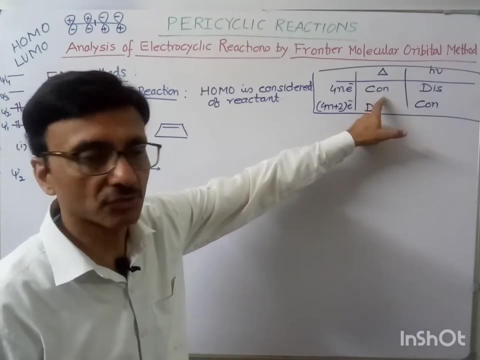 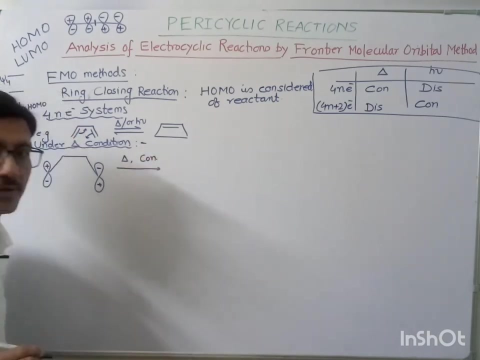 we have to analyze. So this is what type of system. This is for an electron system And under thermal condition, the orbital should undergo Kohn rotation. So let us see whether this undergoes Kohn rotation or not. So if I do the Kohn rotation, what will happen? 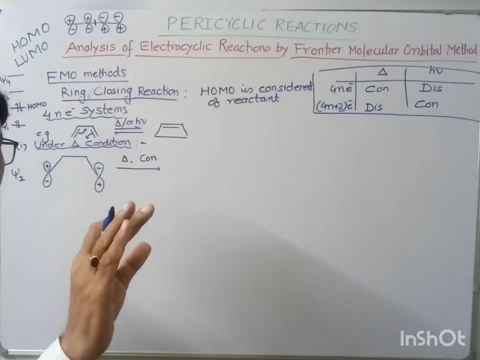 If I do, the Kohn rotation means the orbital are moving the same direction. So this is moving, suppose, in a clockwise direction. This is supposed to be in the same direction, So of course also moving in a clockwise direction. So if this lobe moves in a clockwise direction, 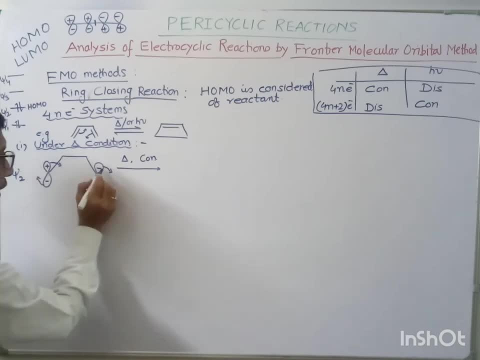 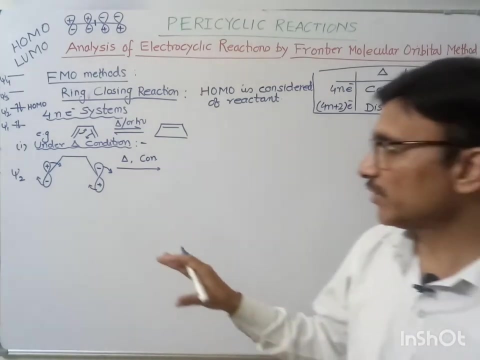 like this, then this will go over here and in a same way, if upper lobe is in this direction, then lower lobe will be in this direction. These both are moving in a clockwise direction. Either we can take both clockwise or both anticlockwise. So if I have taken here both, 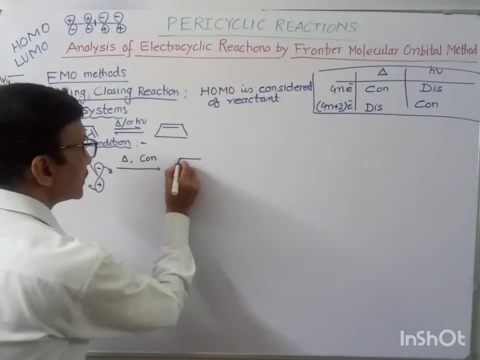 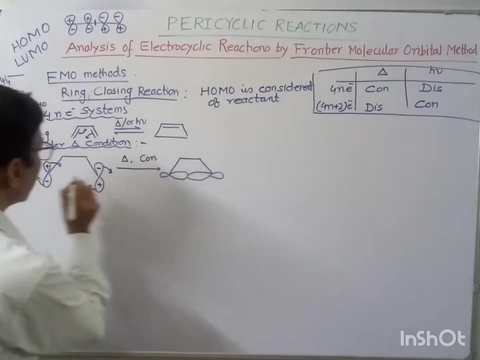 clockwise, then what you will see? You will see that a sigma bond would be formed, and here this will have the positive- This is coming in, positive, This minus lobe is coming going out. This is minus, This is plus and this is minus. So what we have- we can see a interaction here is interaction. 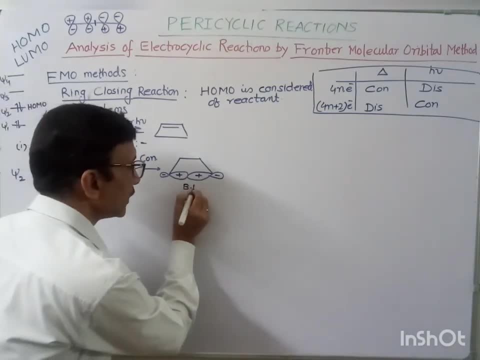 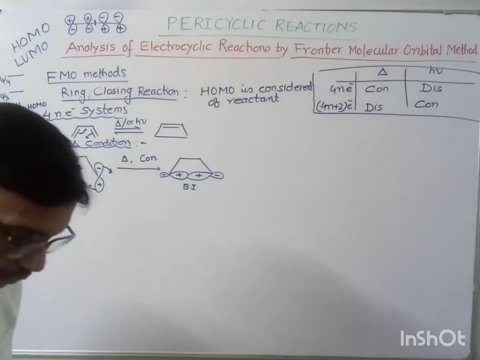 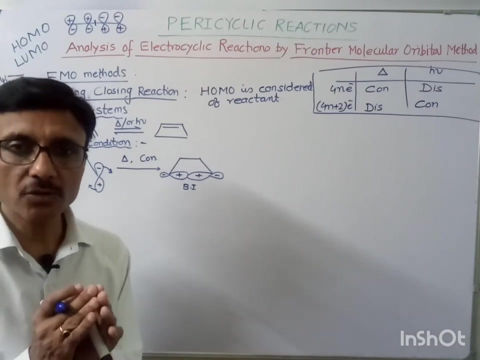 is Bonding. interaction means bond has been formed. It means the ring here is closed. So bond is formed. It means ring is closed, like this And what I have told you: during cone rotation, which type of symmetry should be maintained? C2 symmetry should be maintained during the cone rotation. 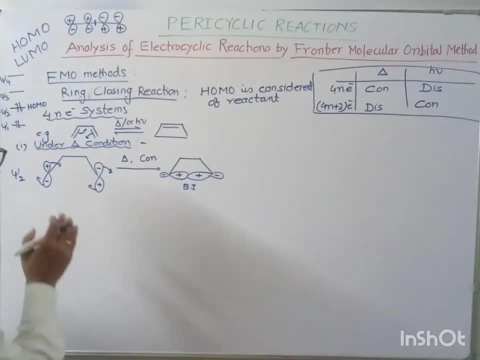 in reactant as well as in product. So let us see whether C2 is maintained over here or not. If one of the rotation axis is dispersed and if rotates it by one, we will have against one another axis. this center axis is again oil-交通. C2 element ratio. 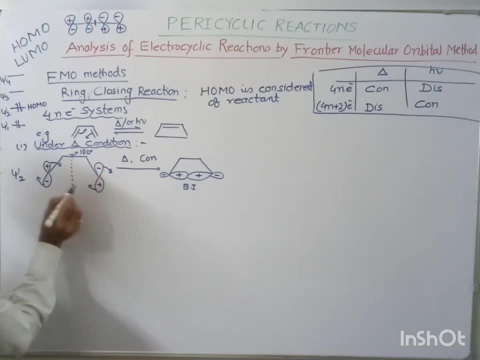 And this is alternative cross gradient or interestingoplanet idea. In respect to this particular case, the rotation axis will be doing체こちら is opposite sideぜひ this S element along by C2 intercrossing когда C1 out of the together is basically: 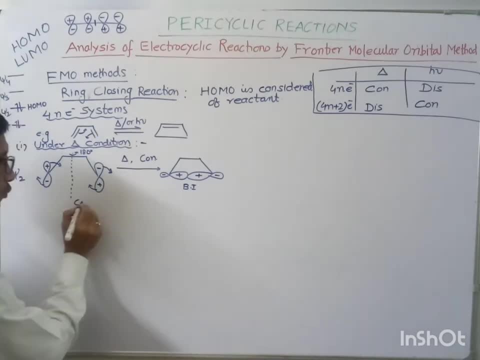 앞에 that is unable to move ahead. So by passing C3 to C4 of the other axis, C3 would come to C4 of the other axis. cans. Okay, So we have here, always according to theliexisteplenia. So what can you do in a kind session In case you wish to see? 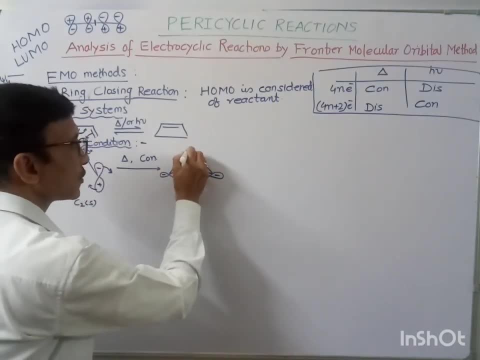 a rotation axis. you can do it with this complicated action, which means let us put seventy-four. If so, here we will see. the direction is approximately okay. Let us not go after that. So now let us do a evaluation of this. 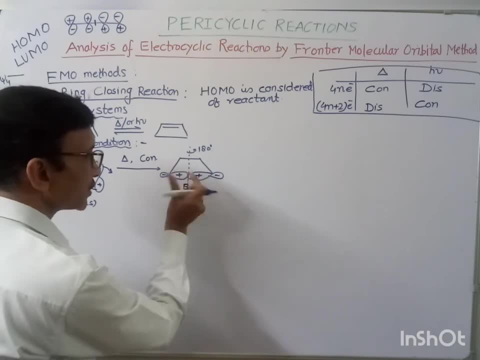 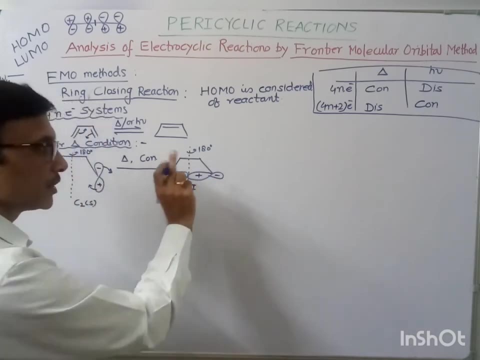 with this pole. this will move in 180 direction, and 180 direction means: at the place of plus, this plus will come. at this place of minus, minus will come. so again here also. it is symmetric with respect to c. it means c2 is maintained. over here it means c2 is maintained. it means this reaction: 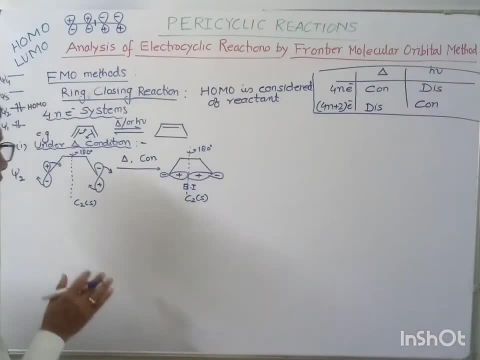 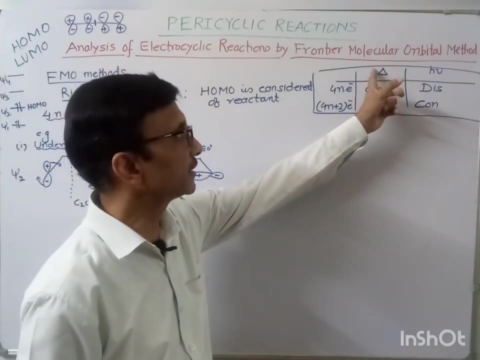 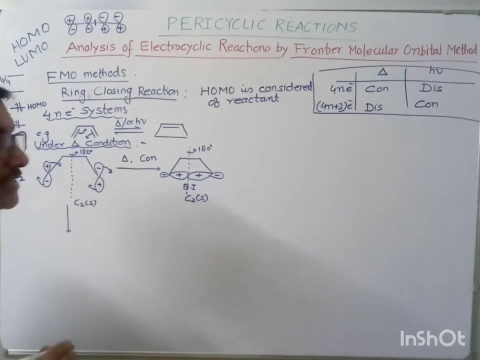 is correct, it means this reaction is correct. so so, under thermal condition, what we have seen, this is analyzed, this is proved, that under thermal condition, cone rotation will occur. now suppose if we, if I do the, suppose I do the this rotation, then what will happen? suppose I do the this rotation. 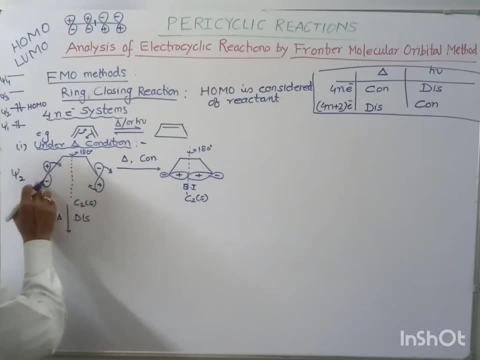 then what should I do? one rotates in a clockwise manner and another. both rotates in a opposite direction. so if it is moving in this direction means clockwise, then this p orbital that should rotate in a anticlockwise manner like this. So what you will see. you will see that so positive is coming here and negative is coming. 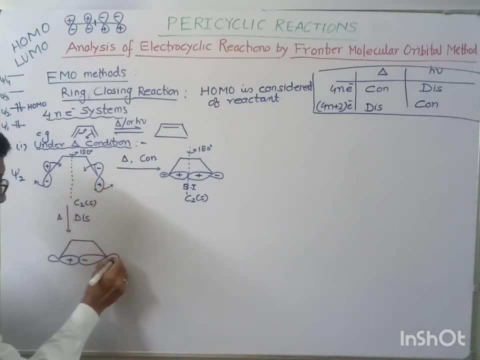 here. so negative is coming here, positive is going on the side, negative is going in this side, like this: what you have seen, what you have seen is positive. negative it means this is showing the anti bonding interaction. so means bond is not formed, sigma bond is not formed over. 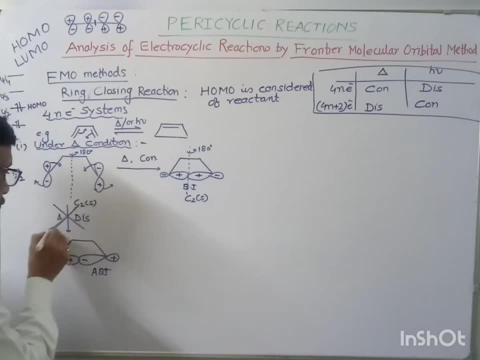 here sigma bond is not formed. that is why this is not allowed. so this is not allowed. and also what I told you during during this rotation: what should be maintained? mirror plane symmetry should be maintained. so here there is no mirror plane, because in front of plus minus is student here. 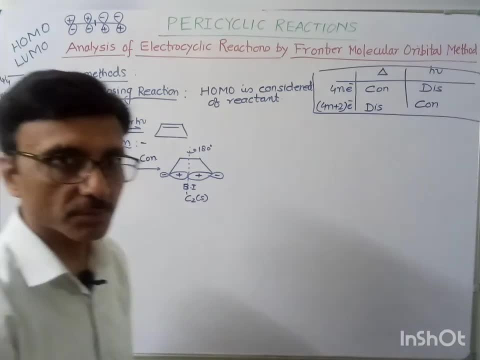 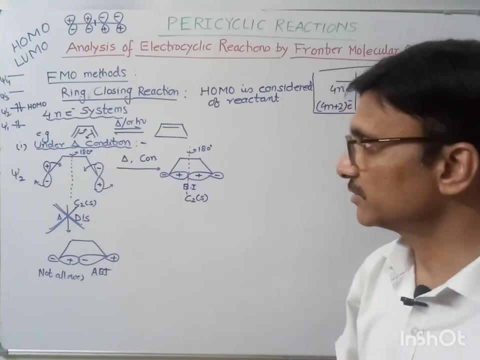 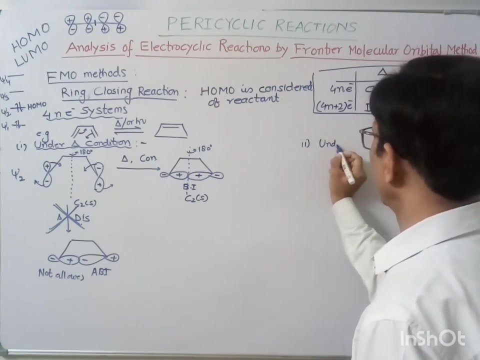 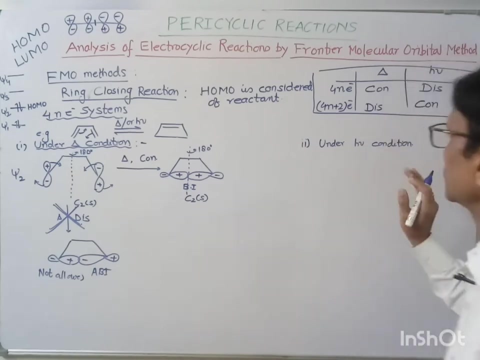 also, the mirror plane is not maintained, so this is not possible. ok, So this is when, under thermal condition, under thermal condition over side, now suppose I take under photochemical condition, under photochemical condition, what will happen? so, according to this rule, what? what is the rule under photochemical condition, this rotation that should takes? 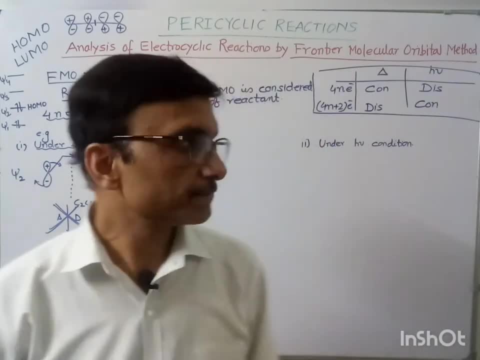 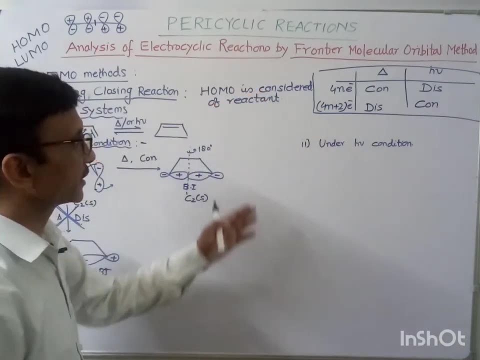 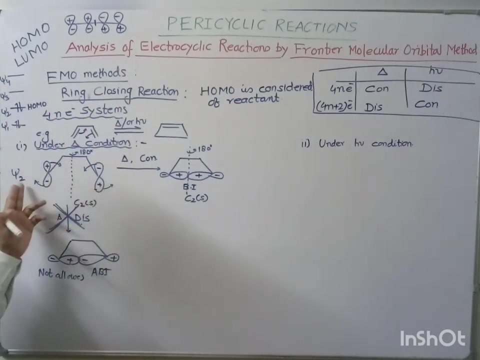 place. So this rotation takes place. so let us see that under photochemical, what we have to see, and in this homo is concerned and considered so for in FMO method, we should take the homo here under thermal condition. homo is side 2. under photochemical condition, what is the? 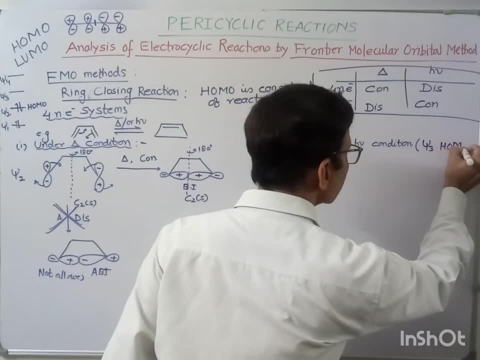 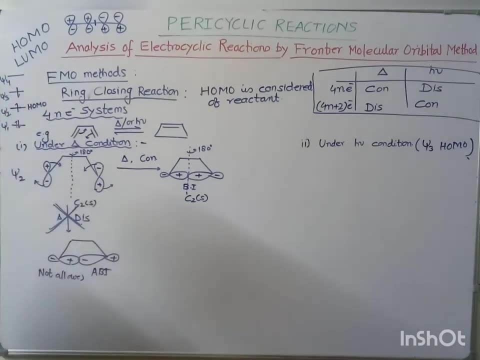 homo. side 3 should be the homo because because one of the electrons from here that will, that will excite it to 2 like this. So that is the homo side 3. that is why this side 3 is the homo here. side 3 is the homo now. 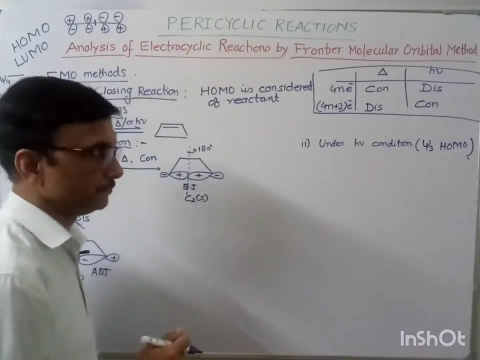 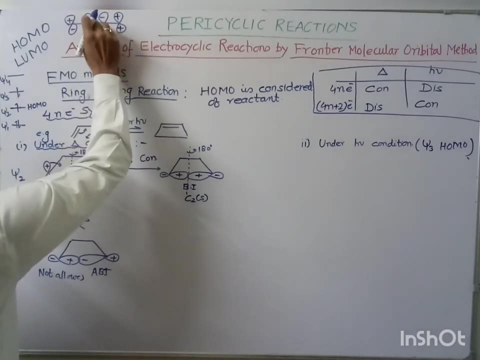 what we can do is: side 3 is the homo. it means what is the sign of side 3? plus minus, minus plus. and in side 3, how many node should be present? 2 node should be present, one node over here, another node over here. so this is our side 3. so this is side 3 and side 3 is: 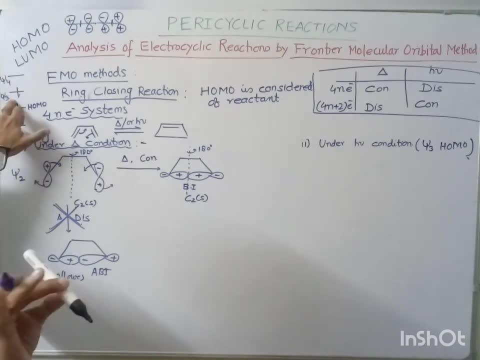 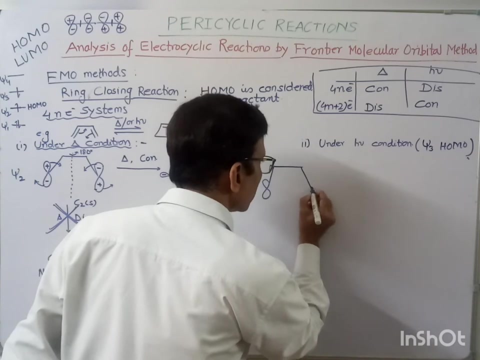 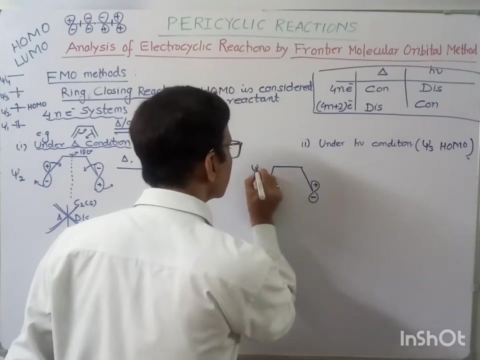 the order. molecular order is the odd molecular orbital. that's why all odd molecular orbital, for all odd molecular orbital, the end orbital should have the positive sign. and we are only concerned with the end orbital. we are only concerned with the end orbital like this. so this is plus, this is our plus, this is minus, this is minus, this is our. 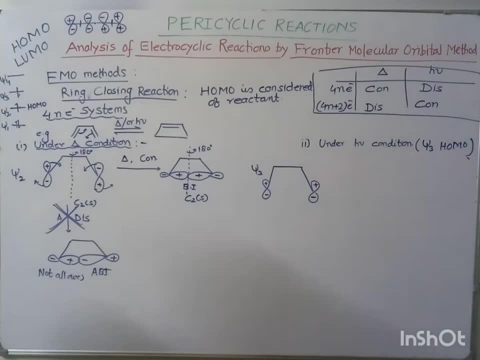 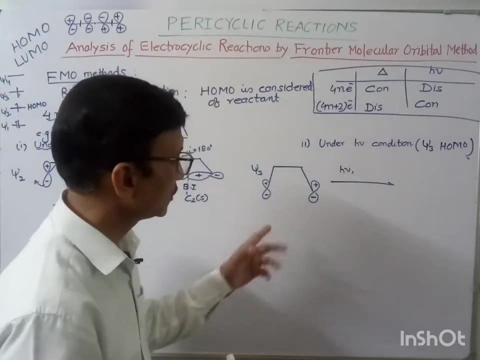 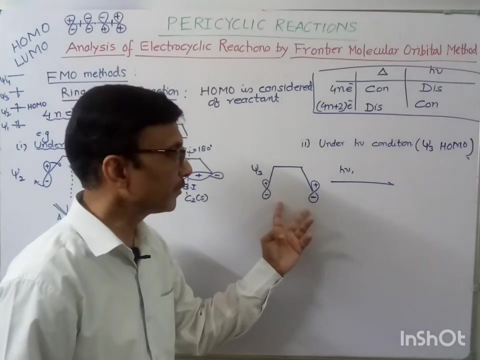 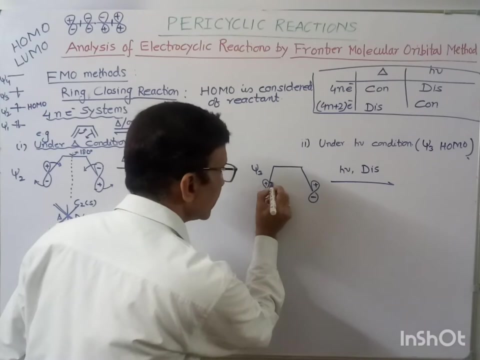 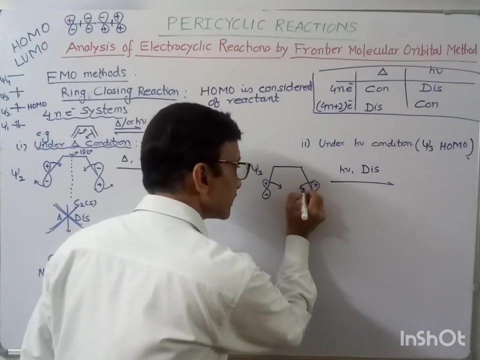 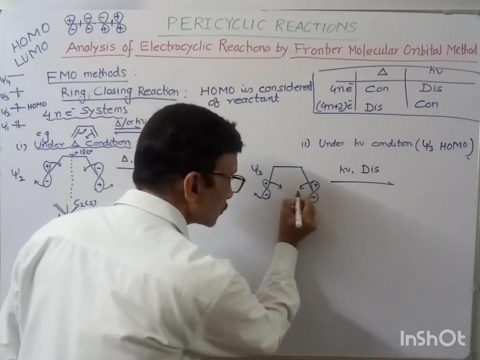 side three. so let us see under photochemical conditions, either they should rotate in the orbital it should go take in a clockwise manner, orbital should go當osaic clockwise manner and another will rotate in a opposite, that is, anticlockwise manner. this is in this direction. in negative loop will go over here if this is rotated in this. 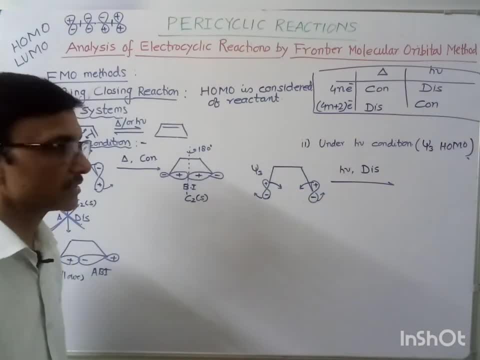 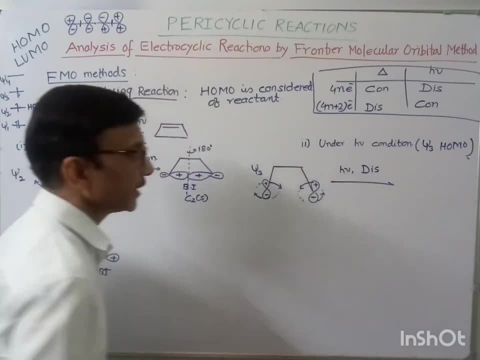 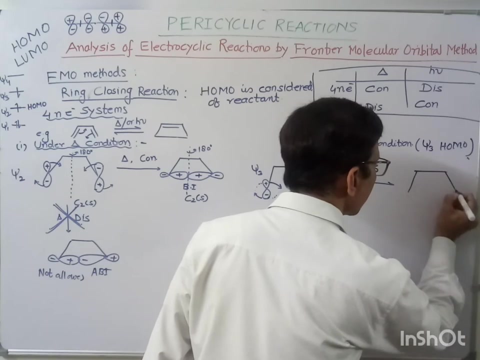 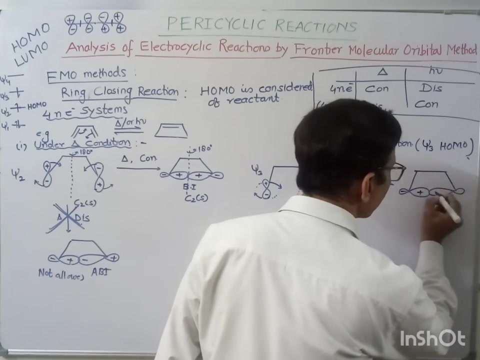 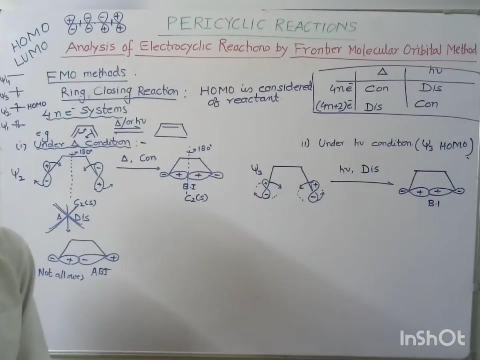 direction, then negative loop will be go over here like this. okay, so what we will see? we can see that it Sigma bond is formed. Sigma bond is formed plus or minus and minus, so bonding interaction is taking place. if bonding interaction is taking place means this is, that is the reaction. 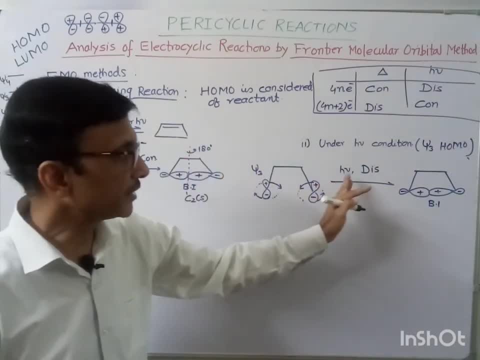 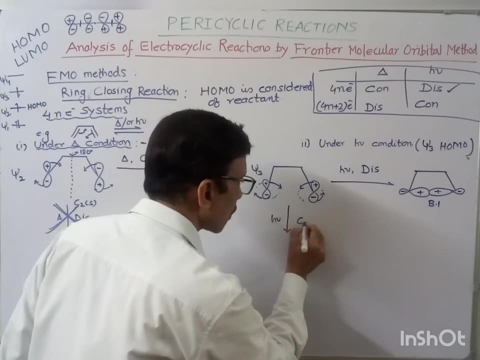 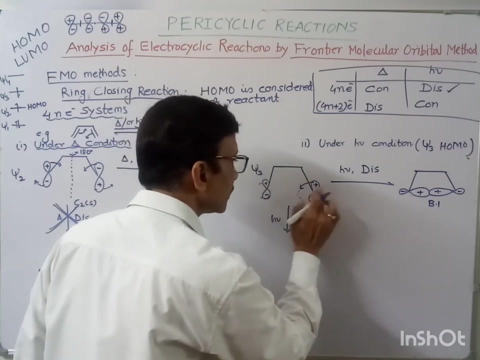 is correct reaction which takes place when under this rotation. now, so this is now has been proved. now, suppose, suppose, if I do the corn rotation, and what will happen if I will do the corn rotation, then what will happen? both should move in a same direction. if this is moving in this direction, if this is moving in this. 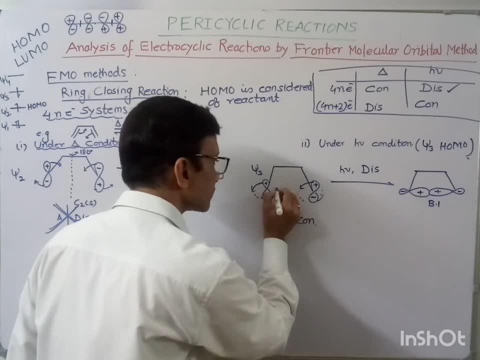 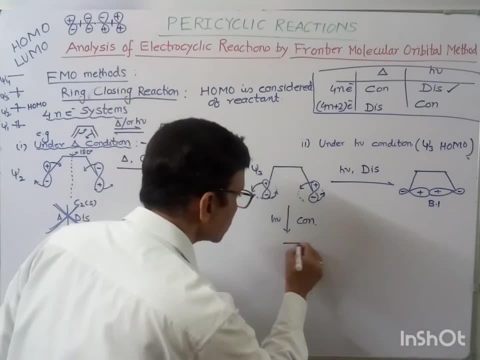 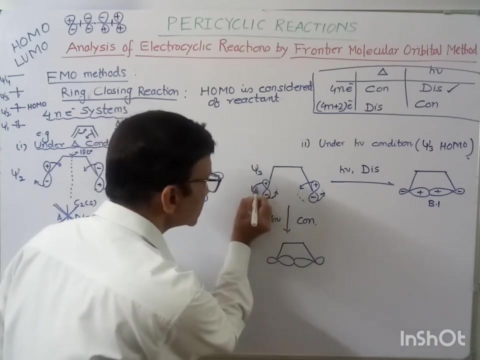 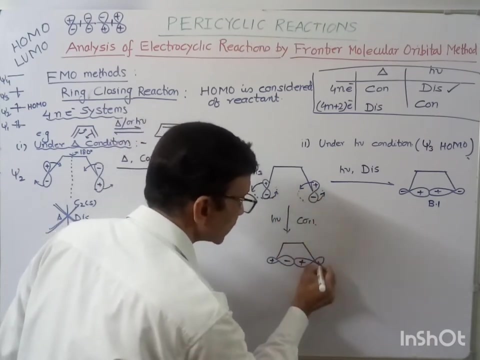 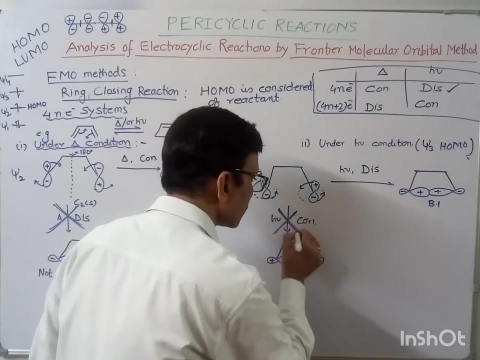 direction. this and this should also move in this direction, like this: okay, this should move in this direction, okay. so what you will see? you will see that. so plus is in this side, minus is in this side. here, plus is here and minus is outside. it means this is anti-bonding interaction and which is not possible. 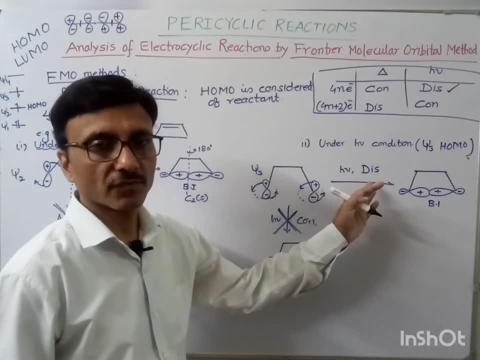 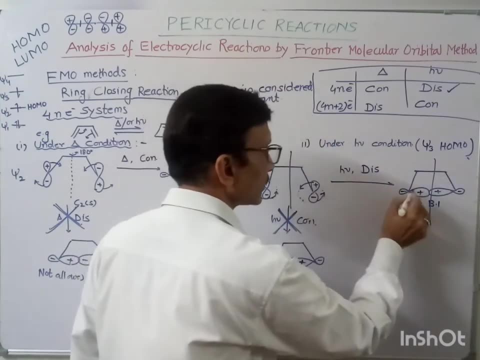 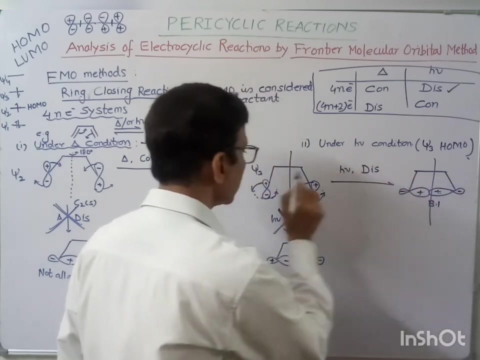 also, if you see in this rotation what symmetry should be maintained, mirror plane symmetry is maintained. so if you will pass a mirror, then what? in place of in the front of plus, you have plus and in front of minus, you have minus. here also, in front of plus, plus, minus, minus, mirror plane symmetry is maintained. 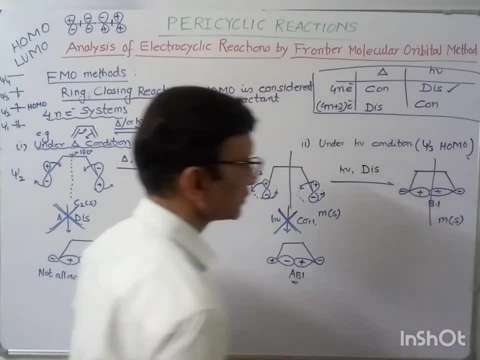 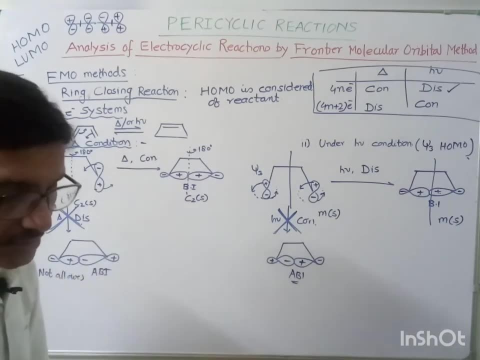 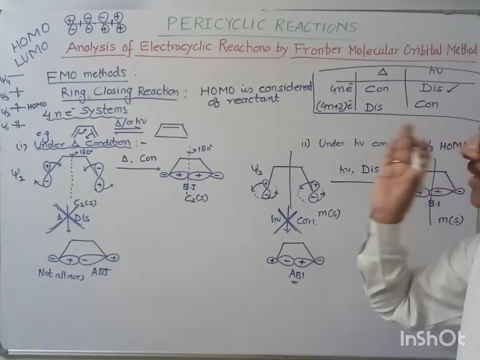 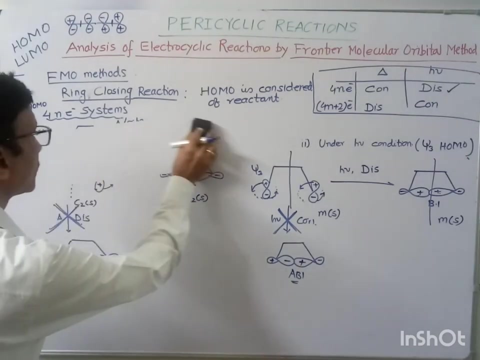 here also, mirror plane symmetry is maintained, sigma is maintained. okay, so this is the way in which we can analyze: the analyze with the help of help of anti-hat molecular orbital method. So this is one of the foreign electron system. in a same way, I can take another foreign electron system. 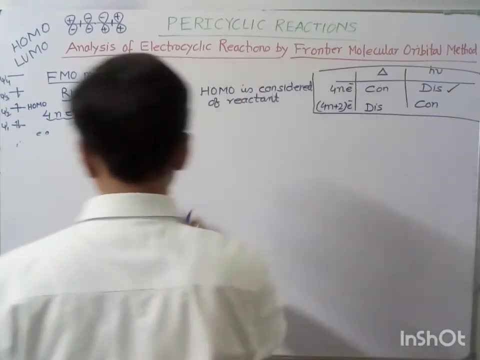 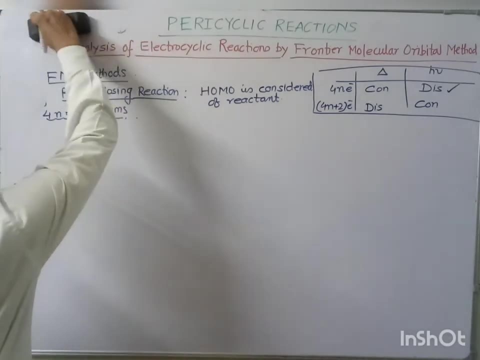 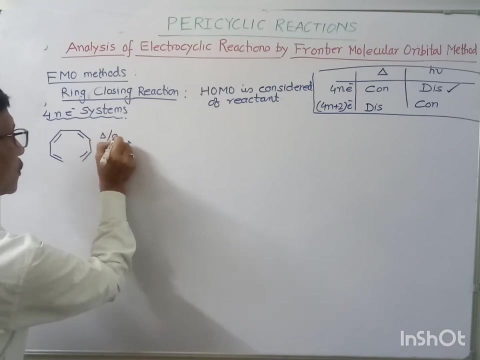 So if I take another foreign electron system then you may have again check and ring closing reaction. again, I am taking the ring closing reaction, So in suppose I take this. Ok, Ok, Ok, Ok. So octa tetra in. so octa tetra in, in presence of either heat or what you will find so a 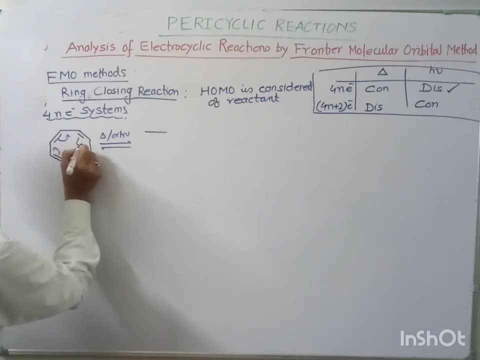 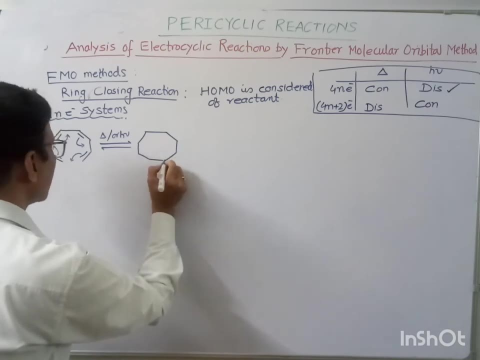 cyclic shift of electron will occur. cyclic shift of electron will occur, and what you will get here? you will get a closed ring. we get a closed ring over here. so this is a ring closing reaction. Now this can also be analyzed, suppose under photochemical condition. 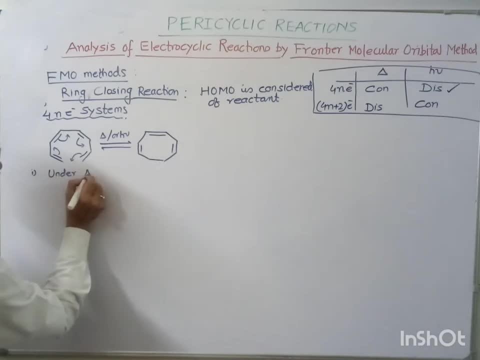 under thermal condition. let us analyze under thermal condition first. So this is also for an electron system. this is also for an electron system. so, under thermal condition, what should be the homo for this? This is: how many pi electrons? 4 pi electrons, 4 p. how many p orbitals, 8 p orbitals. so 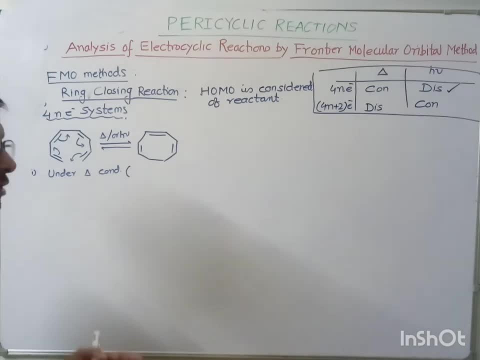 8 p orbitals means 8 molecular orbitals will be there for this. so this will have 8 molecular orbitals: psi 1, psi 2, psi 3, psi 4, psi 5, psi 6, psi 7, psi 8, psi 1,, psi 2,, 3,, 4,. 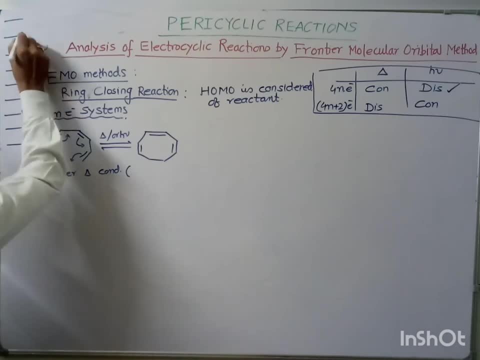 5,, 6,, 7, 8.. 8 molecular orbitals are there. how many electrons are there? 8 electrons, so we have to fill 8 electrons in this. molecular orbitals like this. ok, So what is here Under thermal? 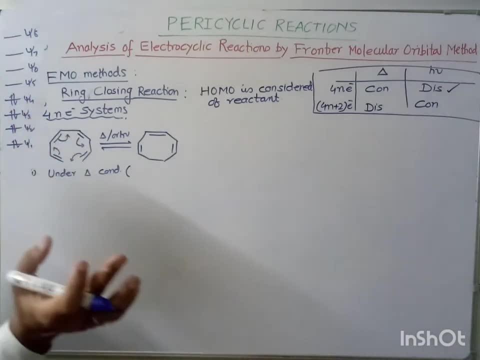 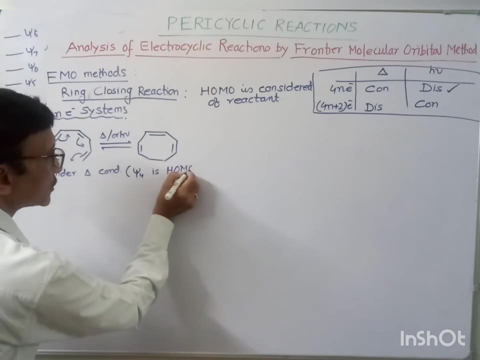 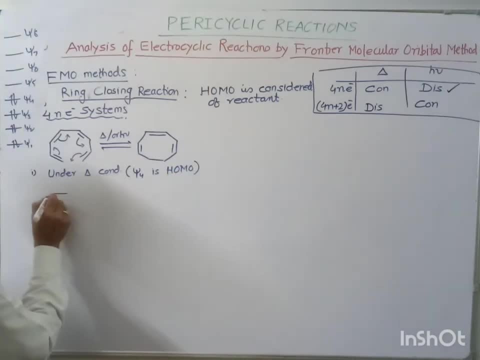 homo. psi 4 is the homo. it means end orbital, because this is even molecular orbital. in case of even molecular orbital, what I have told in my previous lecture, in my previous lecture I have told, the end orbital will have the opposite side. so end orbital, we can draw. 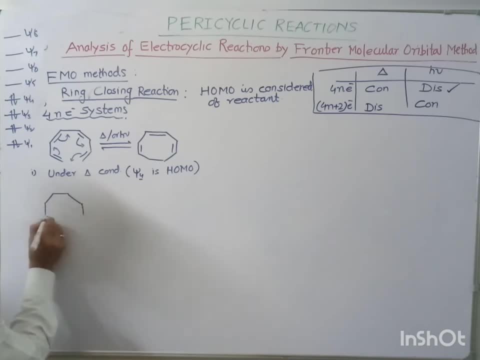 the end orbital. we may draw the end orbital having the opposite side. ok, So if this is in fact minus plus, then this will be minus minus plus. ok, so under thermal condition, suppose I do the pawn rotation In pawn rotation, what should I do? This will moves, both will move in a same direction. 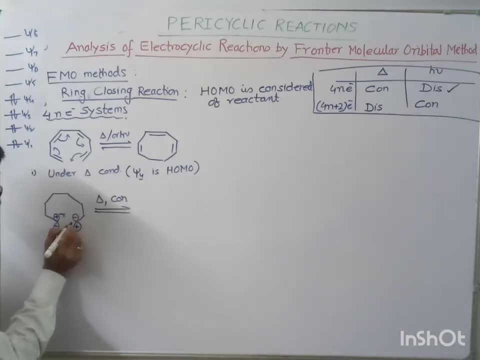 this is moving in this direction, Then then this will also. this will move in this direction. same direction, both orbital will move in the same direction. so if this is moving in this, then this will move in this direction. ie, it shit in the same direction, ok, So 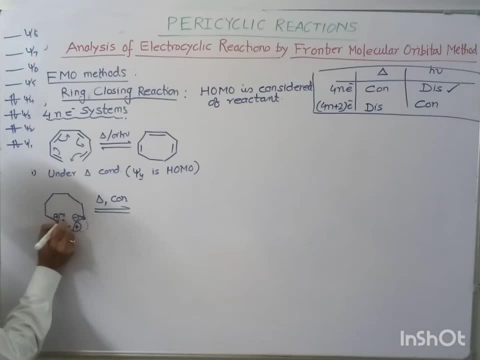 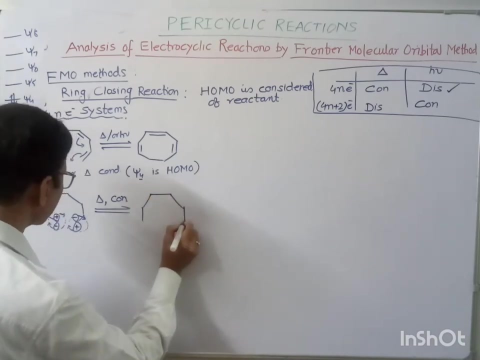 this will move in this direction, like this, and again, this will also move in this direction, like this. So what we will find? We will find that there is a bonding interaction. There is a bonding interaction plus coming inward, and this plus is coming inward. This 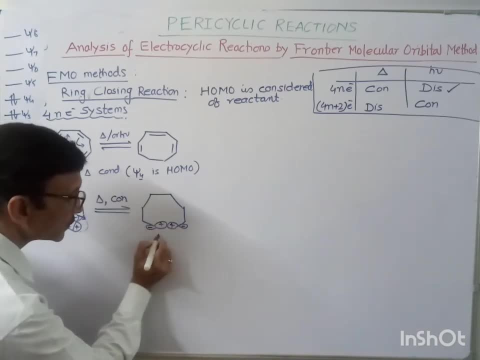 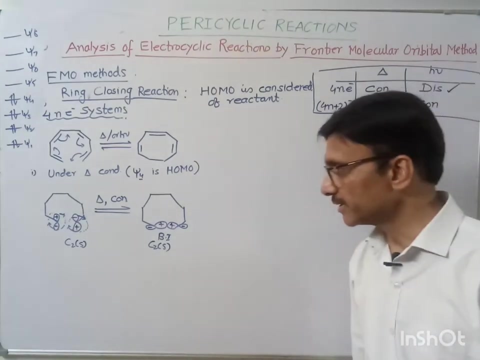 plus is coming inward. This plus is coming inward and we will say bonding interaction is formed and also, if you will see, this has the C2 and this also has the both reactant and product orbitals, molecule orbitals they are, they are symmetric with respect to the 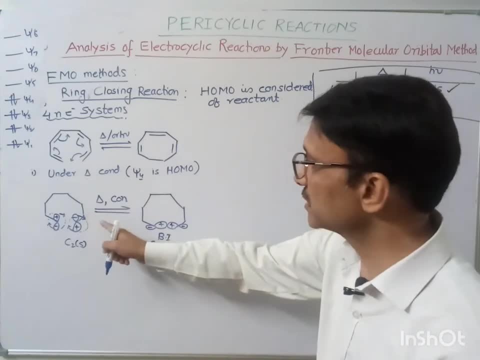 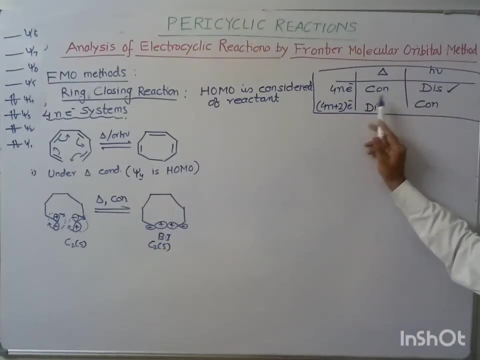 C2.. So again, if you will see, this is for an electron system, this is for an electron system under thermal condition, only corn rotation will takes place, That is, bonding infraction will take place. Now, if you want to do the dis-rotation under thermal, 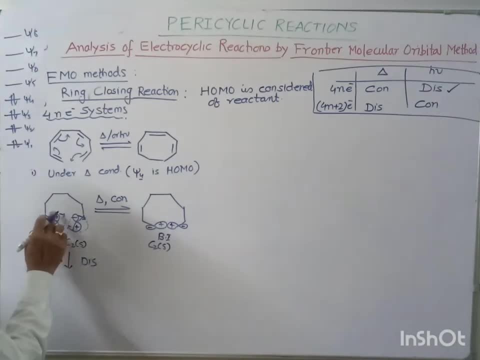 condition. if I do the dis-rotation, then one is moving here and other, then other will move in this direction. okay, So both are moving in a opposite direction. so you will not see any bonding infraction in this case. you will not see. One is plus and this is minus. 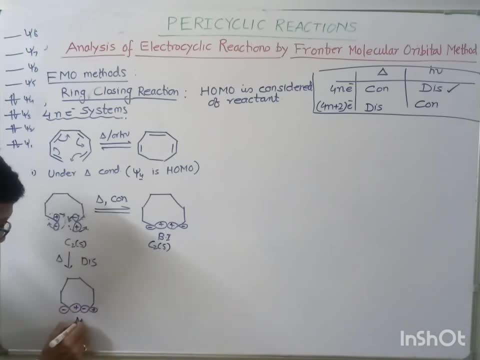 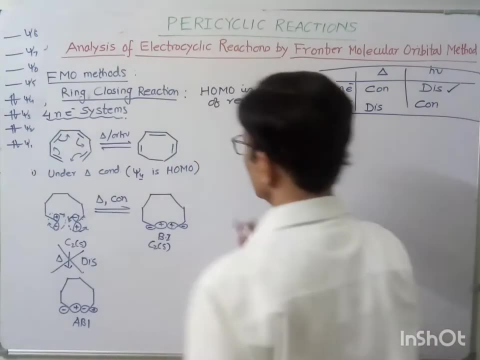 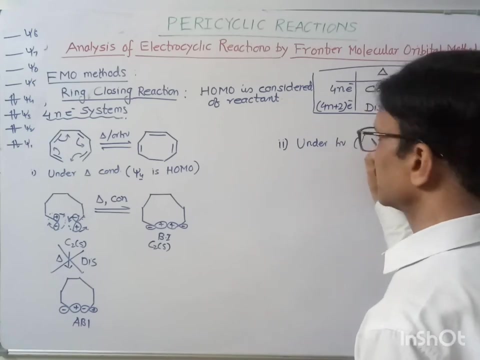 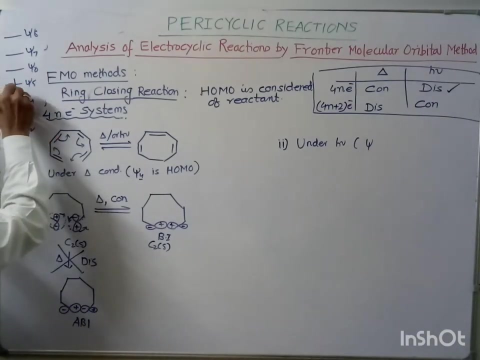 this is minus, this is plus. So this has the anti-bonding infraction. So in the same way we can do for the photochemical condition. Under photochemical condition, what will be the HOMO Psi phi One? electron will get excited over here. It means highest occupied molecular. 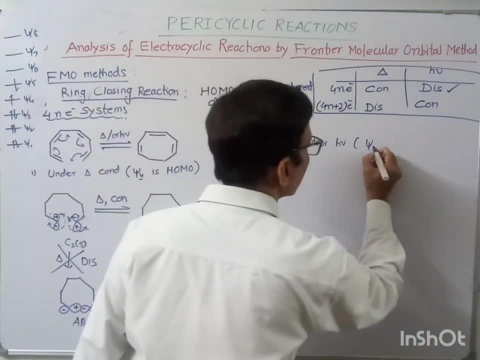 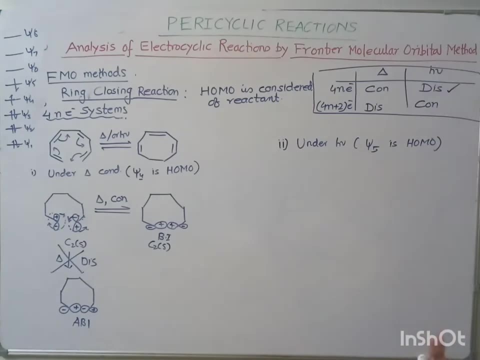 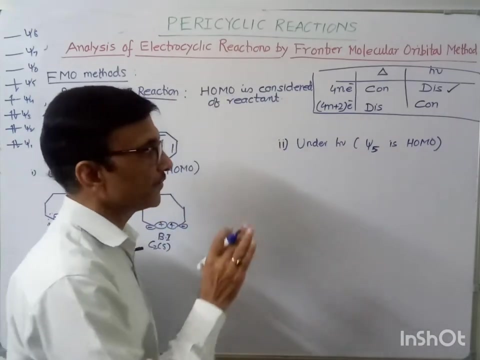 orbital is Psi phi. So Psi phi is HOMO, Psi phi is HOMO. So if Psi phi is HOMO, then what we should write means Psi phi means this is odd molecular orbital. So if it is odd molecular orbital, then n orbital should have the same sign. 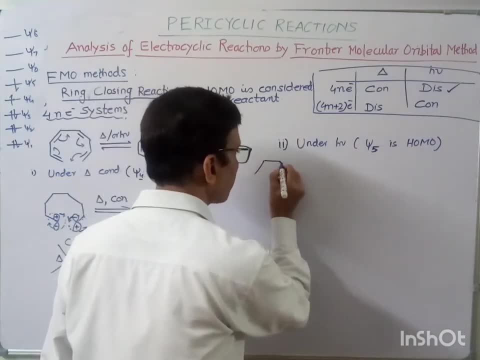 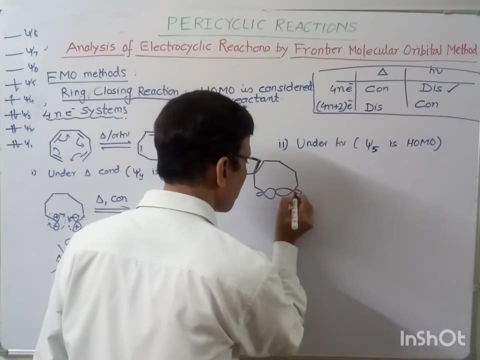 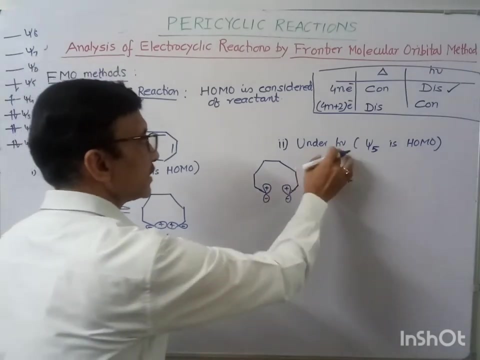 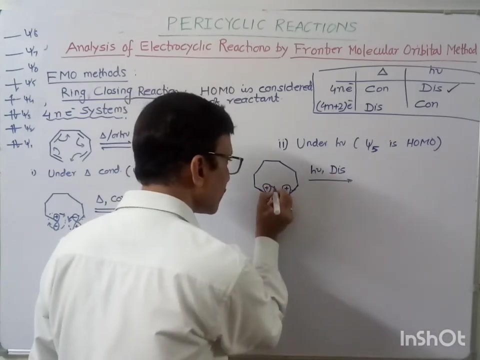 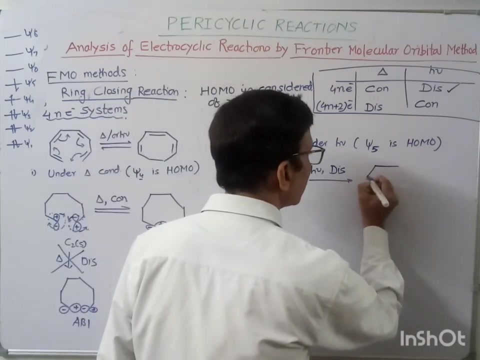 there is positive sign, sure, and orbital positive, positive, negative. okay, so this is under photochemical condition, so suppose I do. the disk rotation means both will move in a opposite direction, like this: both are moving in opposite direction. then what you will see? you will see a bonding. 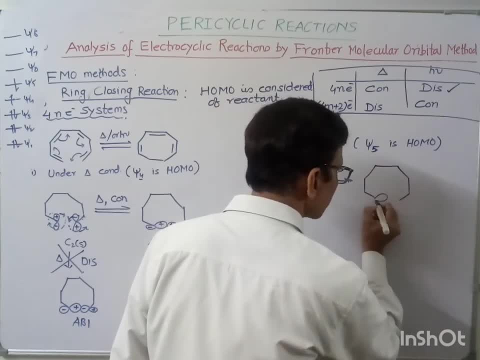 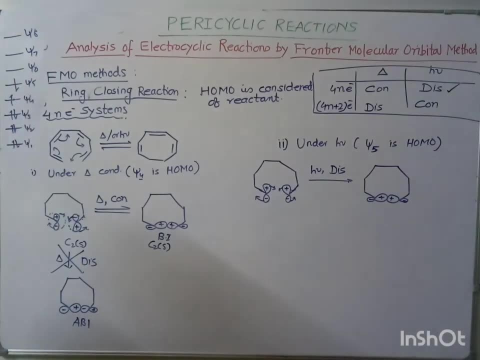 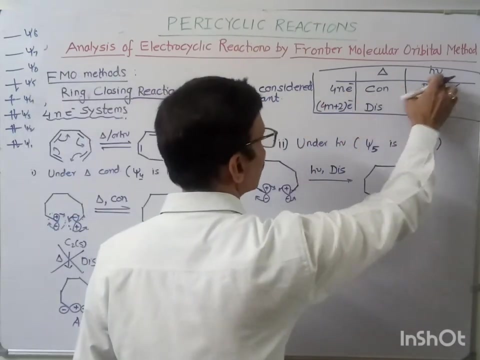 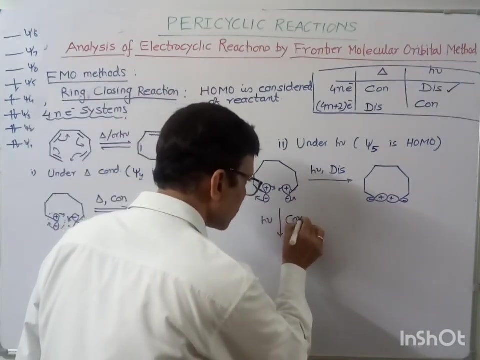 interaction. plus plus minus, this is a bonding interaction. okay, so, as you can see, this is foreign electron system and the photochemical condition bonding interaction. in the same way, if I want to do the con rotation, then in that case we will see the anti-bonding interaction we will see. 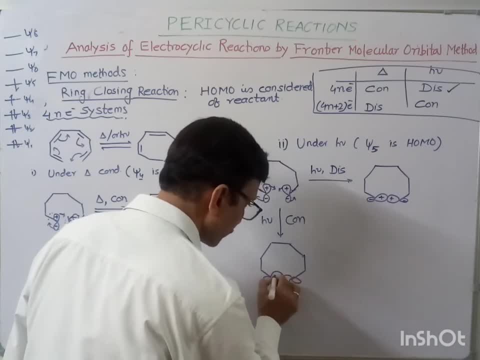 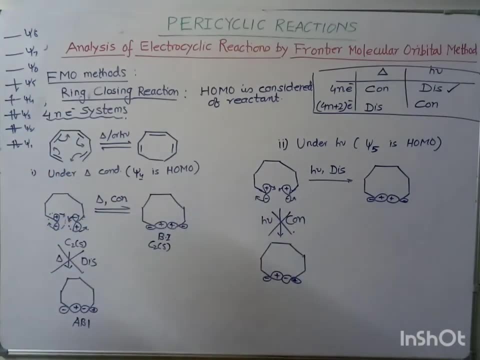 anti-bonding interaction. if this is plus, this is minus, this is minus, this is plus. so this will not take place. okay, so in this way we have seen for 4 n electron system. in a same way let's see for foreign plus two electron system. 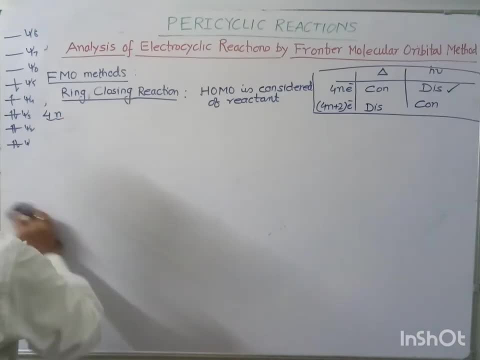 foreign films electron system we may take the example of are trying so on. in presence of heat or light, ring closing will take space. one double bond is coming over here. so this is the foreign plus two electron system and we can analyze this foreign two electron system under thermal condition. this rotation will take space. 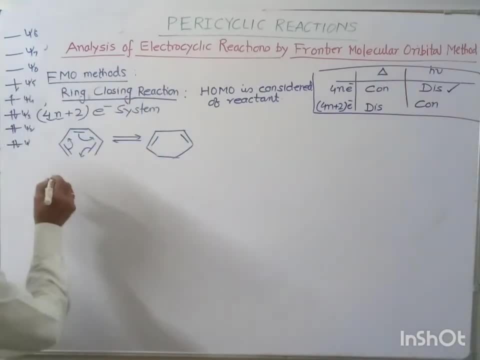 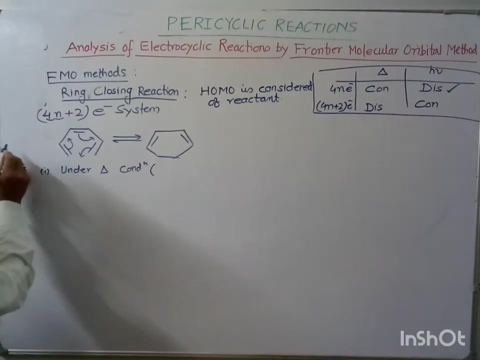 this is the rule that we have to prove. so if you take, suppose, under thermal condition, under thermal condition what would be the HOMO NULL X prime X Kart computer B N, half bonding, okay, so 6 electrons of six, five electrons are there. X, we should fill the 6 pi electrons in these molecular orbitals like this, so this: 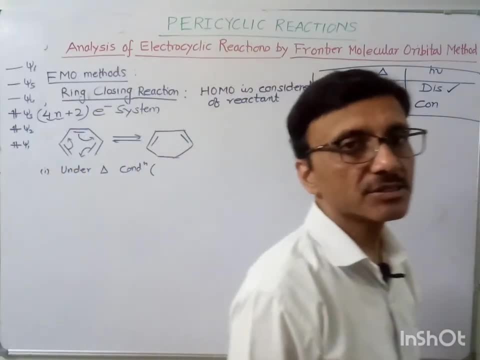 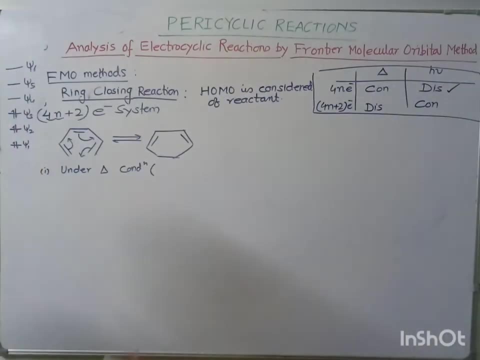 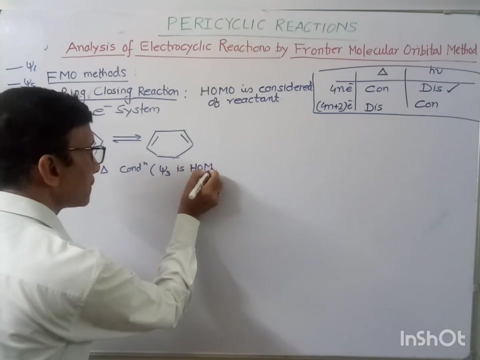 Psi 3. this is the homo. Psi 3 is the homo for your 4m plus 2 electron system. so Psi 3 is the homo and if you will see, then this Psi 3 is the homo. if Psi 3 is the homo, then what you will see: 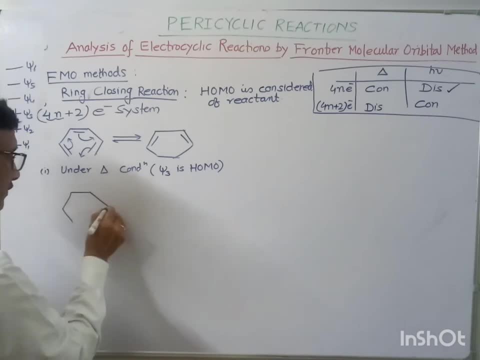 and orbital should have the which sign, positive sign. this is odd molecular orbital. that's why and orbital will have the positive. this is positive, this is positive, negative. now suppose under thermal condition. we are studying in the thermal condition. if we do the suppose pond rotation, what will happen? if I do the pond rotation? then it means both. 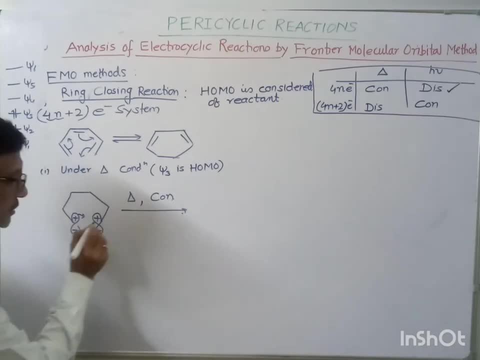 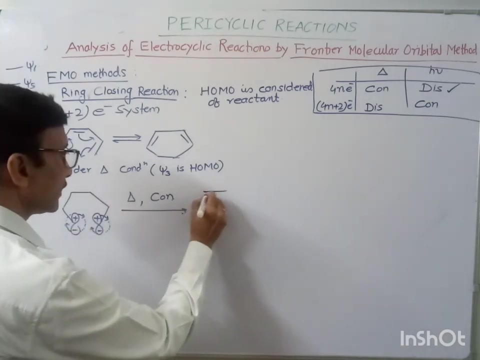 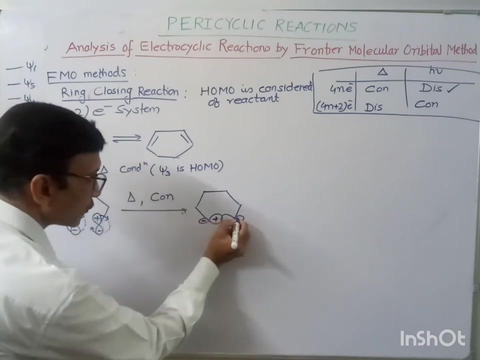 orbital are moving in a same direction. this is clockwise and this is also clockwise. this clockwise, then, this lower lobe that will move like this and this lower lobe that will move like this. so what you will find here, this plus is coming over here. this minus is going over here. this plus is coming. 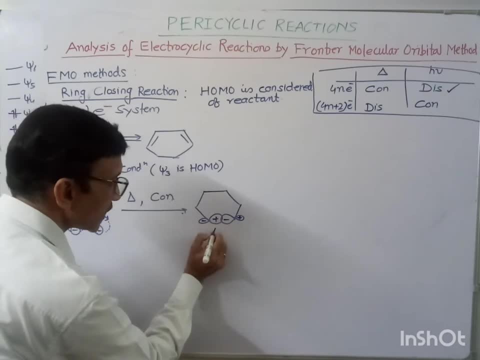 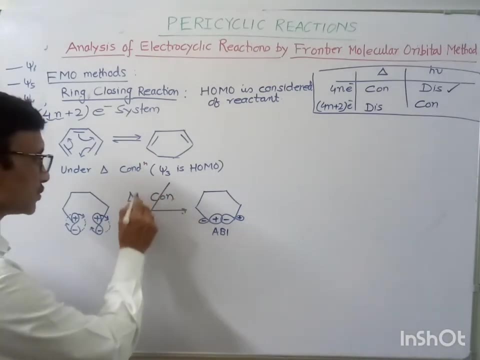 over here and this minus is going over here. so this is anti bonding reaction. bond is not formed means in closing, reaction is not taking place. so this is not allowed, so this is disallowed. whereas, if you will see, if I do this rotation, if I do this, 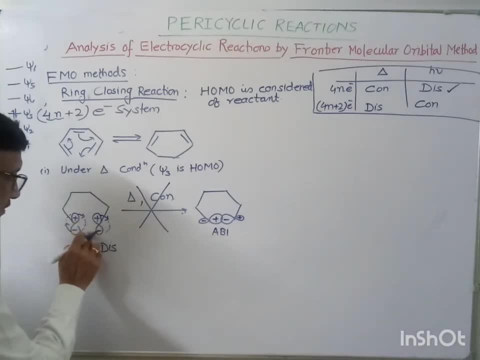 rotation means one is moving like this and another, another is moving, but is moving in clockwise direction, and another is moving in an anti clockwise direction. so what you will find? so this plus is coming in. this is coming in. minus is going out. minus is going out. plus is coming in, minus is going out. this is bonding interaction. this is bonding interaction. 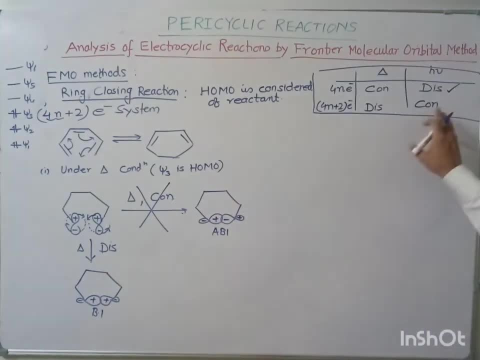 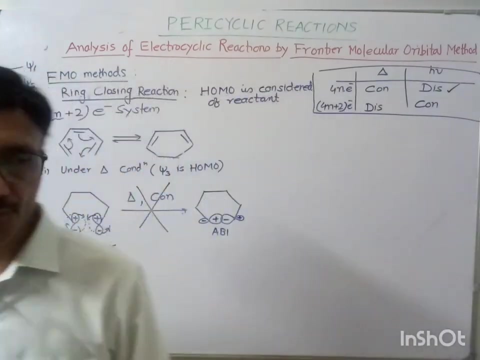 means ring closing is possible when this rotation of orbitals takes place. so under thermal condition ring closing. ring closing is only possible if the orbital rotates in a disrotatory manner. so this is the first case. now under photochemical condition. let's see in the photochemical condition. 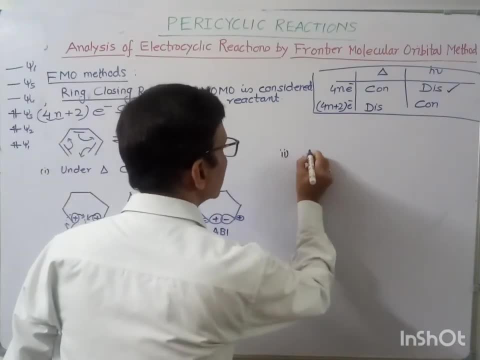 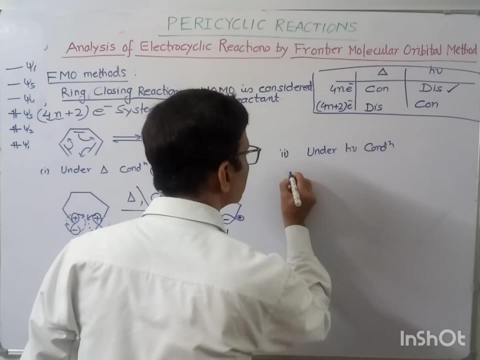 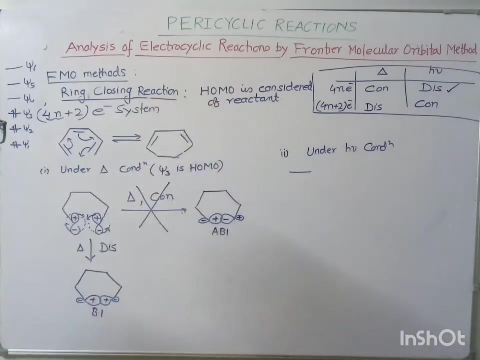 this is under thermal condition, so under photochemical condition. see then what will the homo on the photochemical condition? so we have to consider the homo, we have to consider the homo. homo under photochemical condition will see, then one of the electron will excite to here and now. psi 4 would be the highest, or куп När. 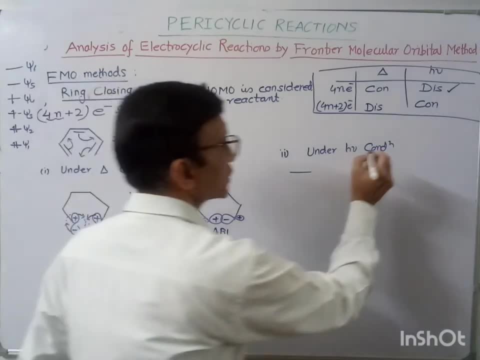 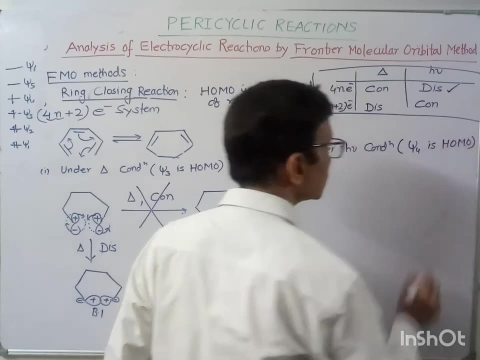 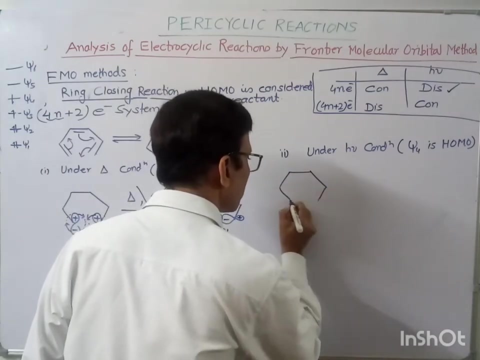 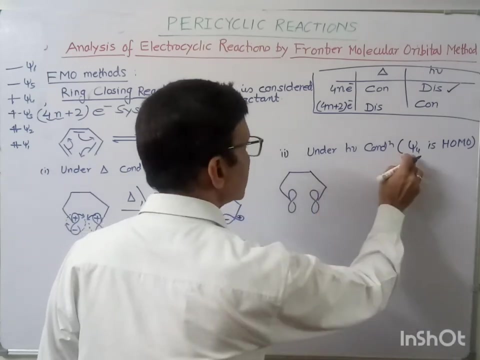 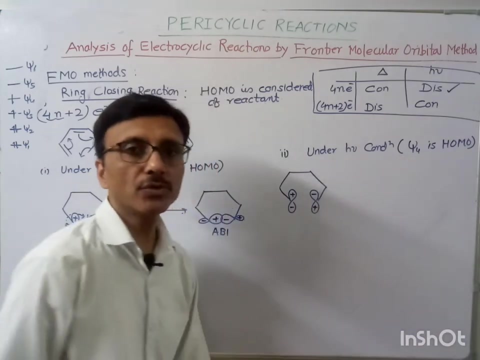 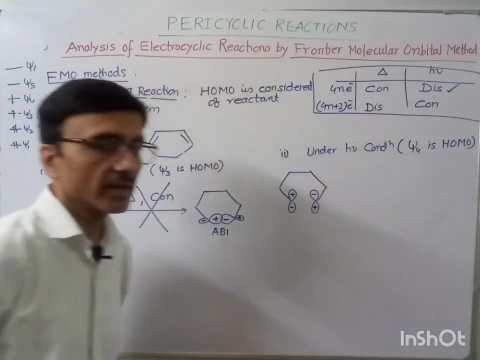 compassed electron, Chris, molecular orbital. So here psi 4 is highest occupied molecular orbital. So if this is plus, this is minus, this is even molecular orbital. So what I told you, for even molecular orbital and orbital should have the object's time. So like this, and what we can do if 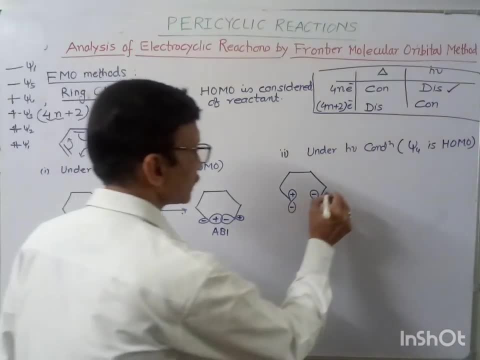 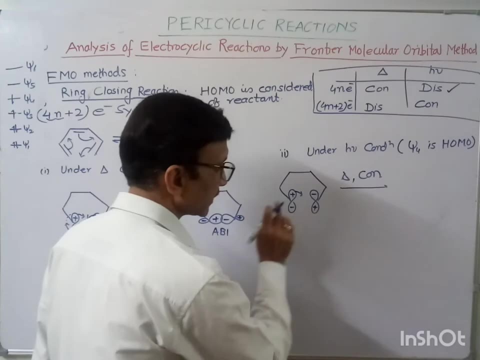 I do the suppose. if I am doing the con, rotation means both orbitals move in a same direction. If this is moving in a same direction, then this is moving in a same direction, So this is moving in a clockwise direction. this also moves in a clockwise direction and lower lobe. 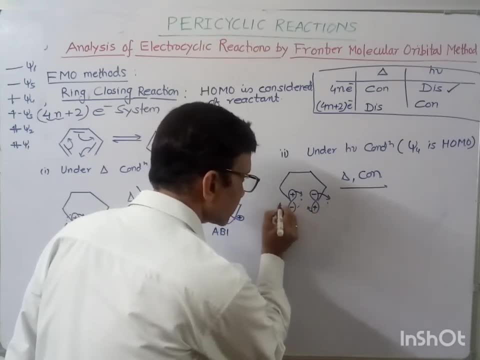 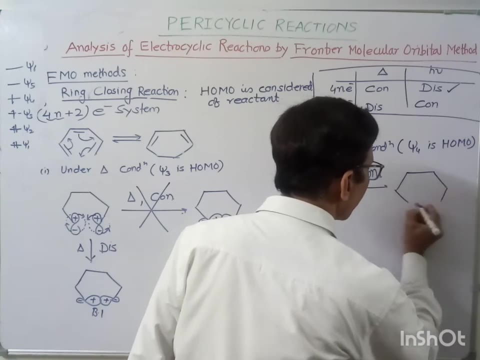 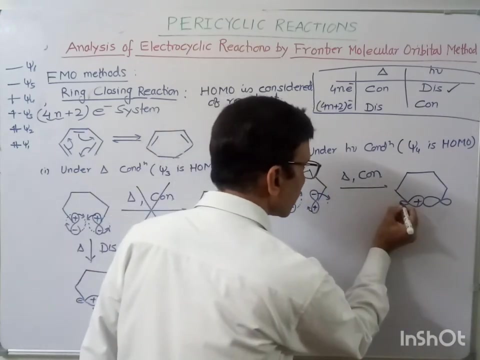 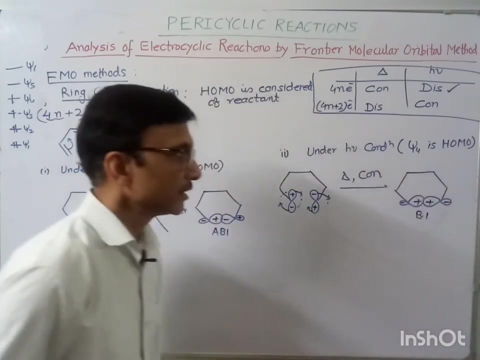 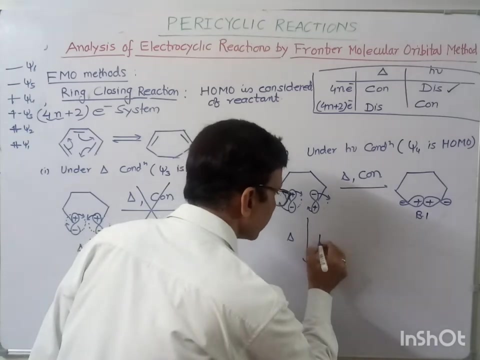 will move like this and this lower lobe will move like this. So what you will find? So plus is coming in, minus is going out. minus is going out, plus is coming in. this is bonding interaction. So this is possible and if I do this rotatory more in this rotatory, both will move in a 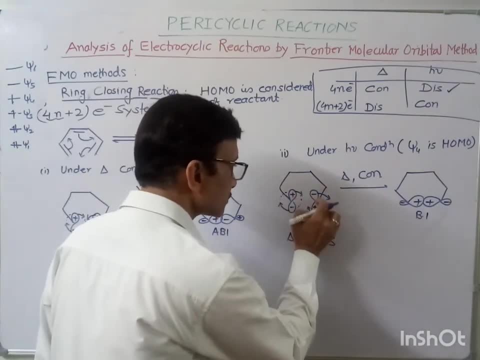 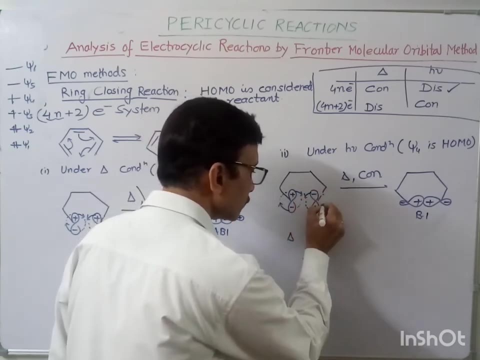 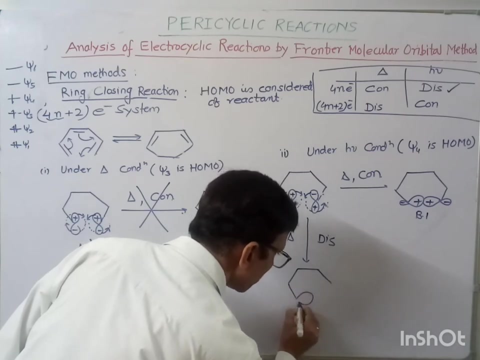 opposite direction. If this is moving in a clockwise direction and this p orbital will move in an anticlockwise direction, means this will move like this and this will go anticlockwise direction in this rotary. So what we will find? We will find this one. Now, this is a anti-clockwise direction and 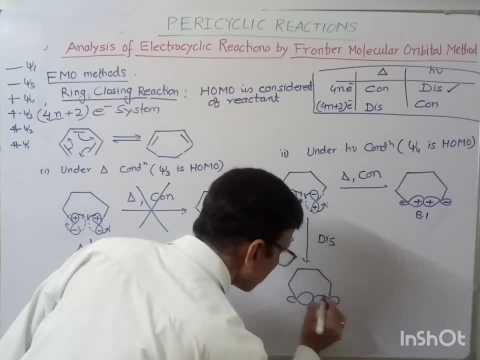 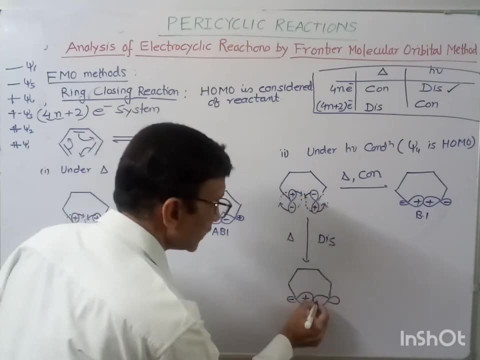 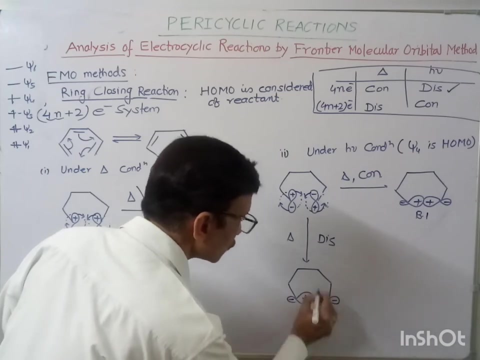 this will move in a anticlockwise direction. Ellie says this will also do that. So how? So this is moving over here. negative lobe is going over here. negative lobe is now coming in. this positive is going outside. so, if you will see, there is anti-bonding interaction. 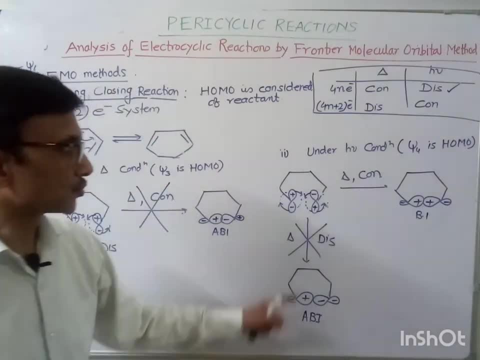 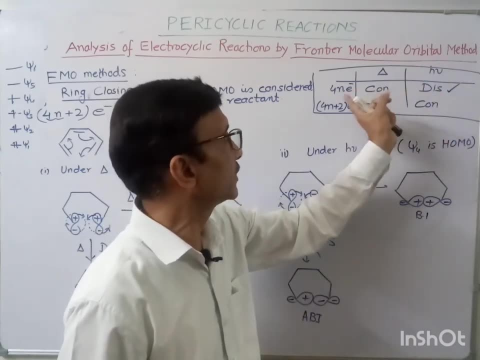 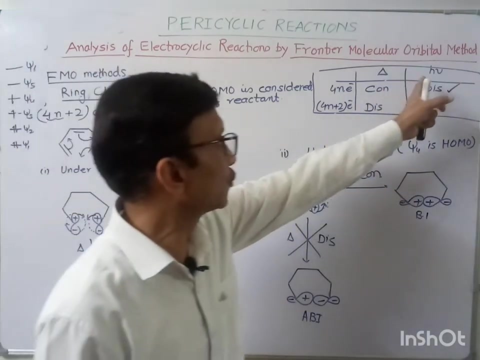 so this is not allowed, bond is not formed. So under thermal condition, what we have to prove for foreign electron system under thermal condition, foreign plus 2 electron system under thermal condition, this is desorbitry. under photochemical condition, this is condom, like this. 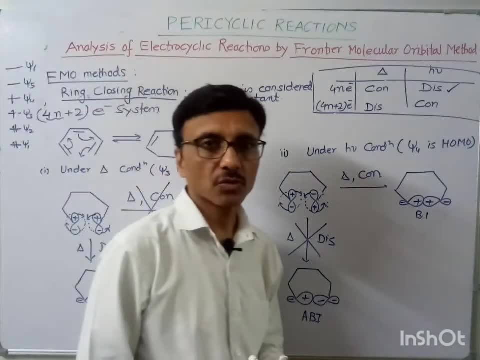 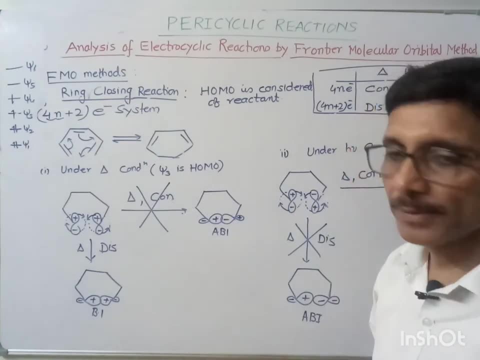 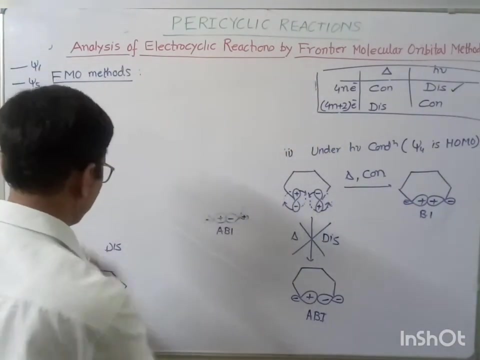 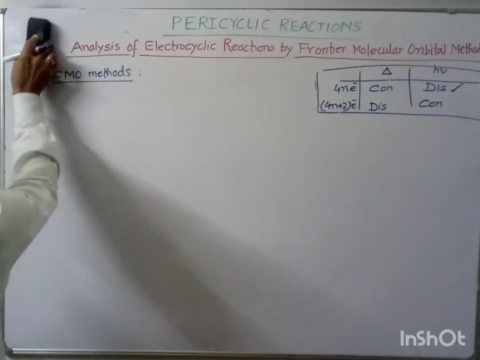 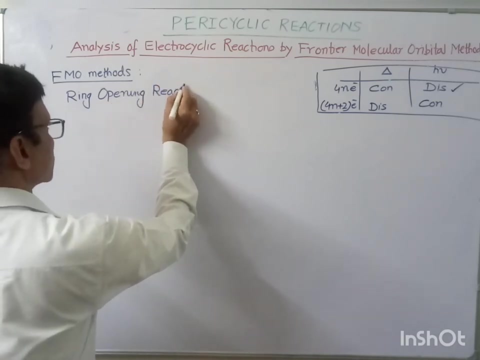 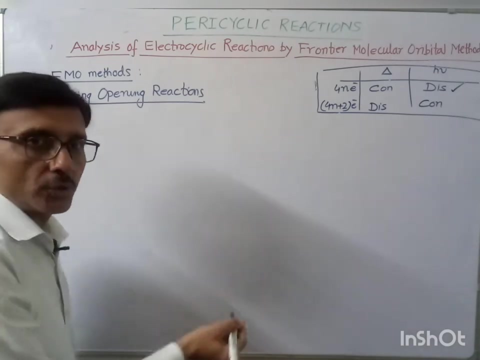 So in this way we may take other examples also. Now we will see the ring. this is the ring closing reaction. now we will see the ring opening reaction. Ring opening reaction. what I told you in ring opening reaction, I will take the reaction. 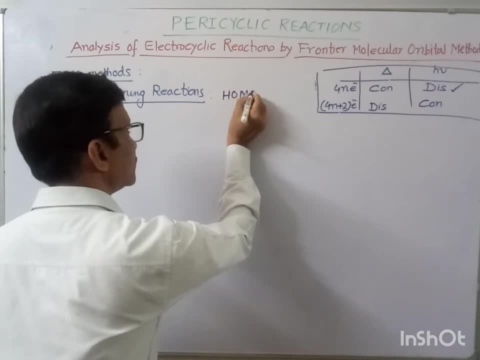 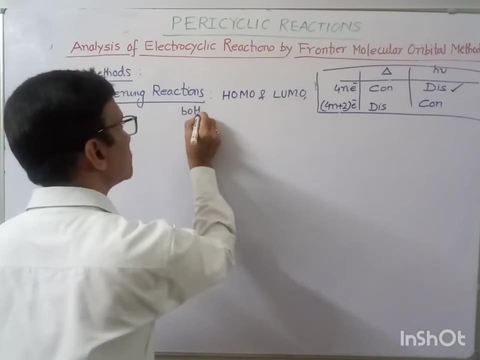 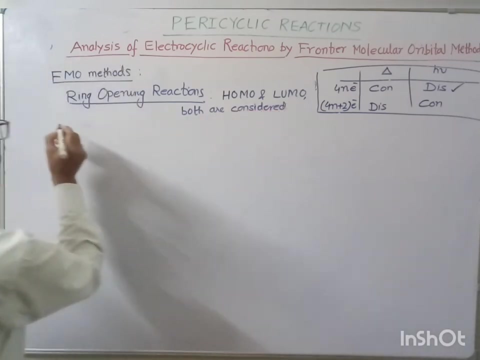 of the electron. take HOMO and LUMO. both are consider HOMO and LUMO, both are considered how? let's take example. so first I will take 4n electron system. 4n electron system, so ring opening reaction. this is our 4n electron system. 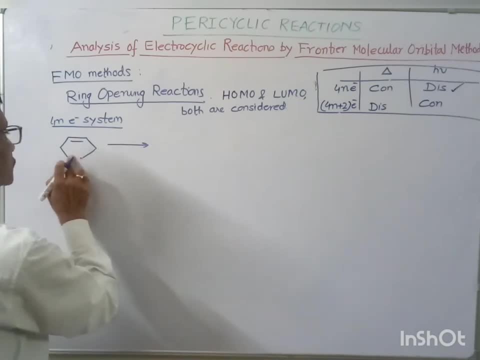 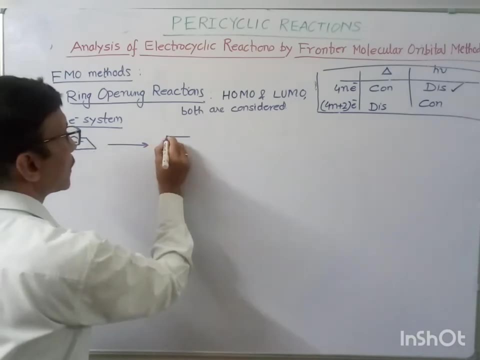 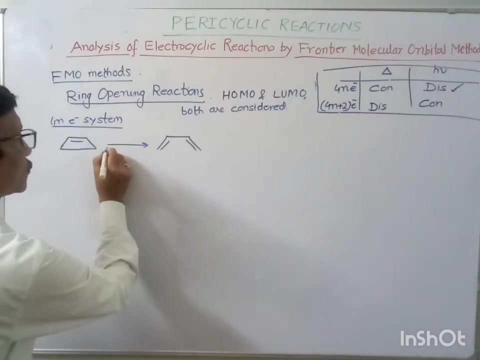 cyclo cyclo butene, it opens into butadiene. so this reaction will occur either in presence of heat or in presence of light, so by the bond rotation of orbital or by the disc rotation of orbital. so, in this case, how we can analyze this reaction? 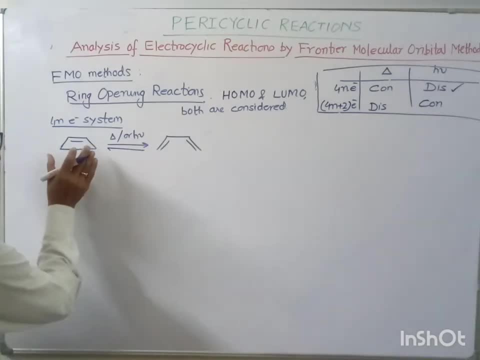 how we can analyze this reaction, how we can analyze this reaction, how we can analyze this opening reaction. so we have to see the reactant. we should see the reactant and in reactant, if you will see, then the reacting, the reacting partner is one- this sigma bond- and another, this pi bond. 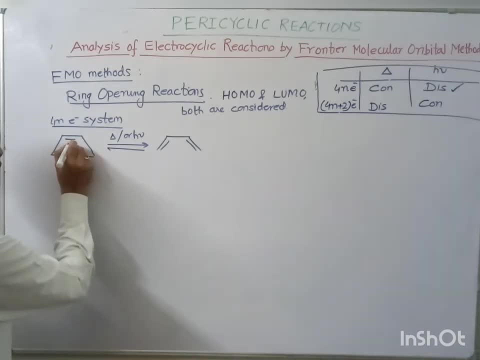 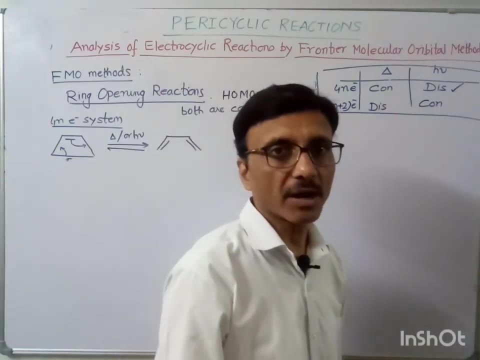 because here this will go over here after absorbing the heat of light, and this will go over here. so sigma bond and this pi bond, these are the reacting part. so sigma bond and this pi bond, these are the reacting part, or we can say this is the two reacting partners. 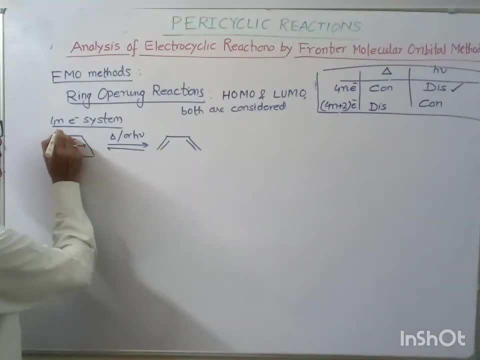 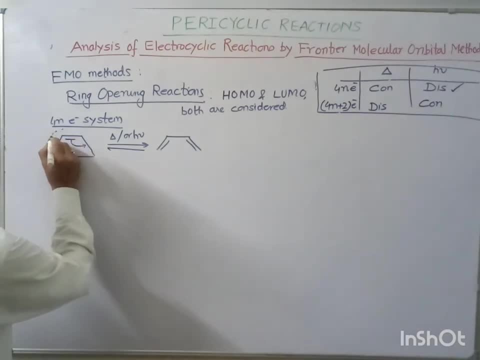 and another reacting partner and another reacting partner. this is the another. sigma bond is the another reacting partner. so two reacting partner is there. so two reacting partner is there. so two reacting partner is there. so first reacting partner is the pi bond. pi bond is the first reacting partner. 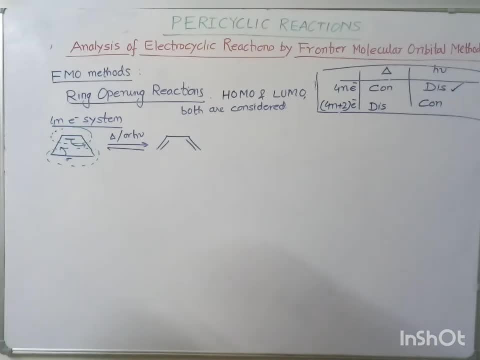 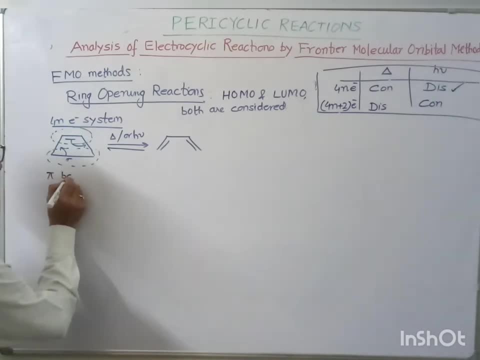 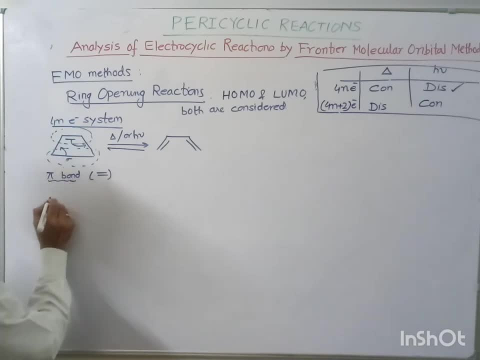 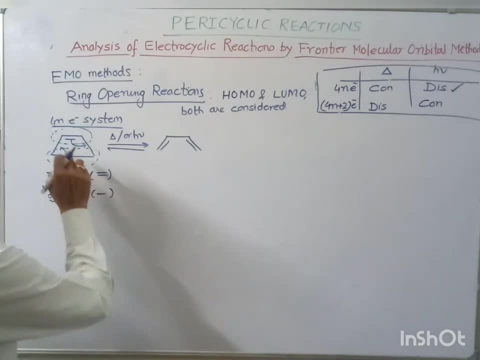 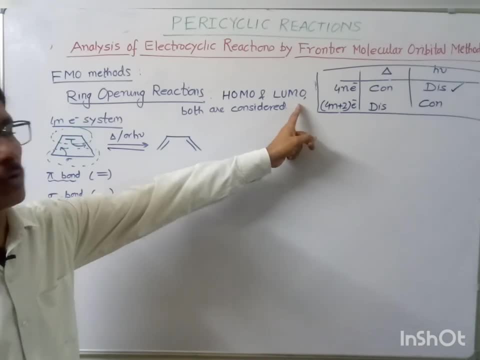 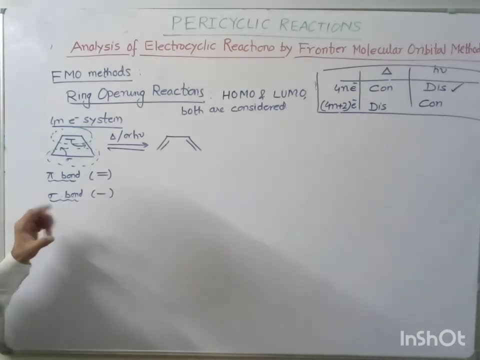 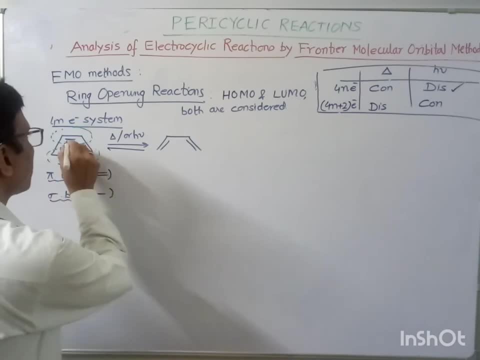 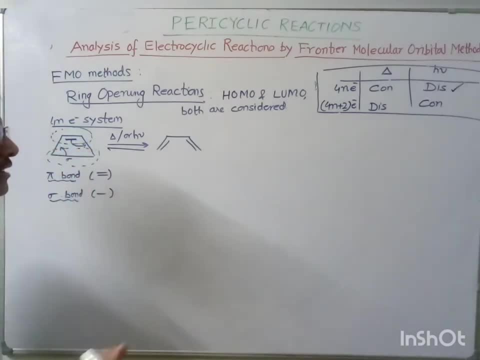 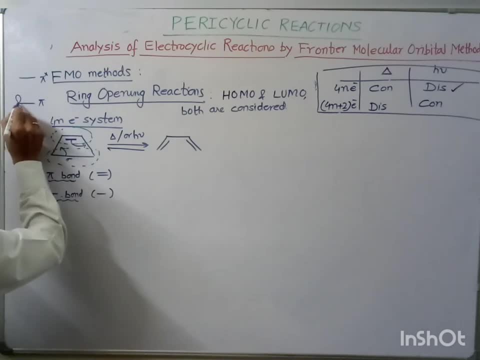 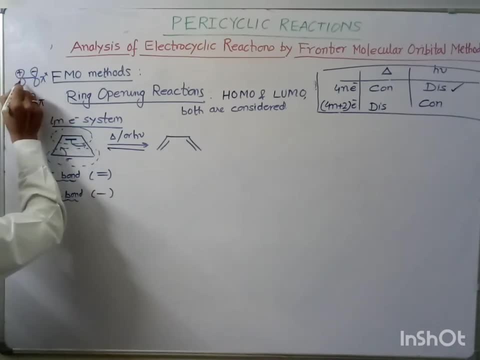 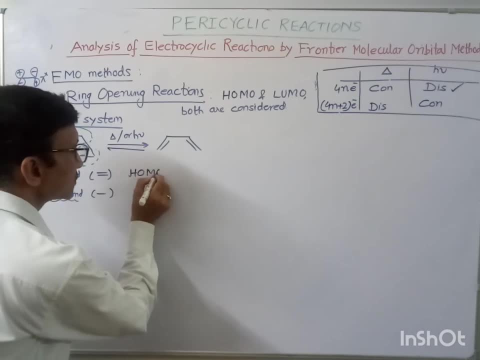 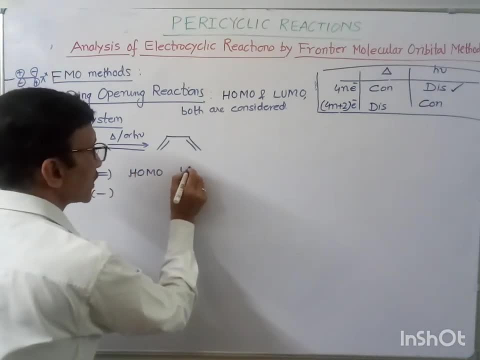 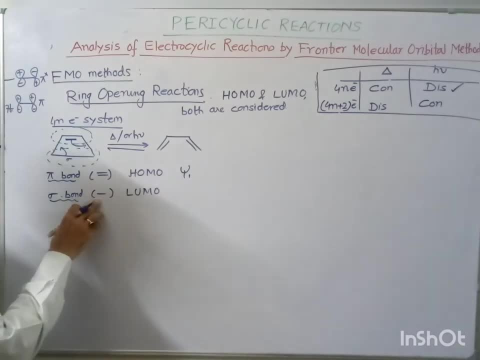 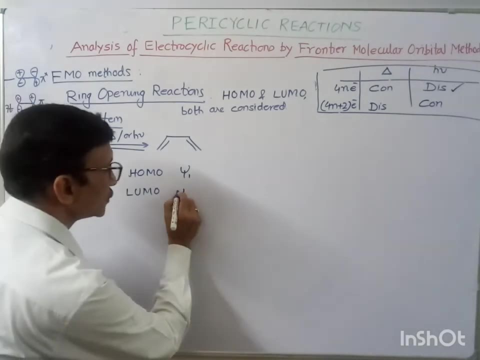 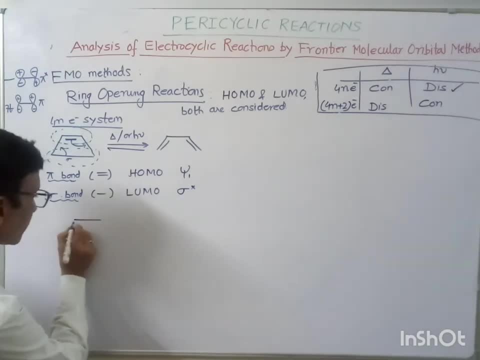 Now what I will see. Now let us see. So I should take the HOMO that is psi 1 of this pi. Psi 1 of this pi is plus, plus. So this is one reacting partner. I have taken HOMO. 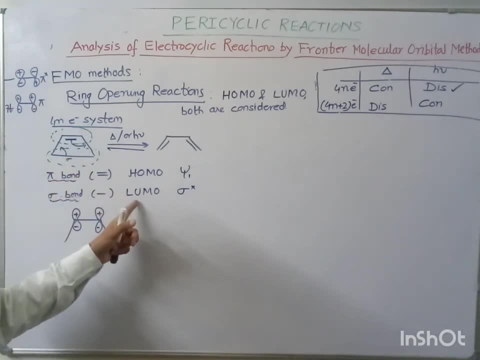 plus, plus. And for sigma bond I should write this: sigma star. So sigma star is here, This is our sigma star. One sign is plus, another sign is minus. This is minus, this is plus, Like this, Now, let us, this is opening reaction, This is being opening reaction, Now under. 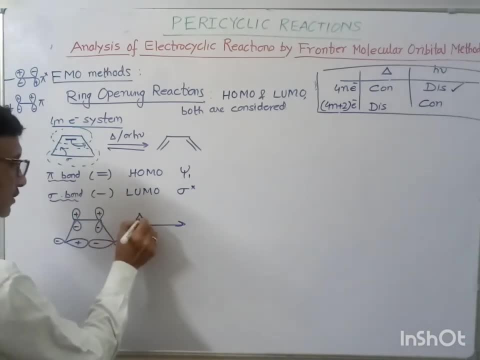 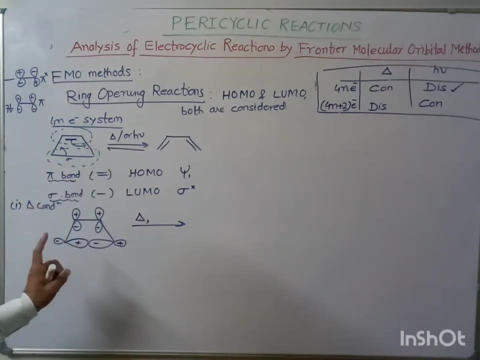 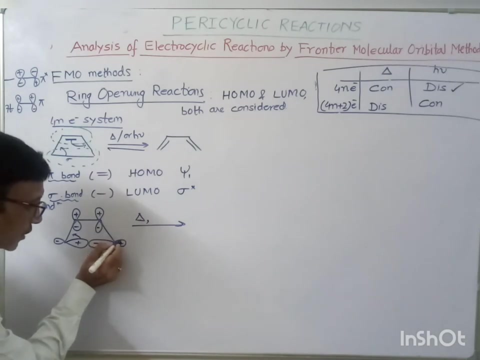 suppose thermal condition under thermal condition First is under thermal condition, So under thermal condition, suppose I open. it opens in a con-rotatory manner. So in a con-rotatory manner means if this is anticlockwise, then this orbital will also move in an anticlockwise. 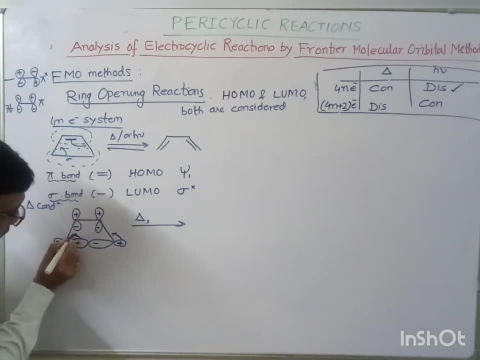 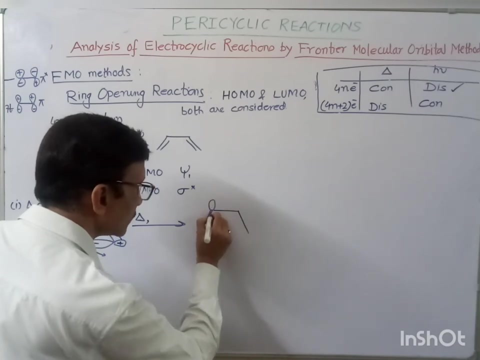 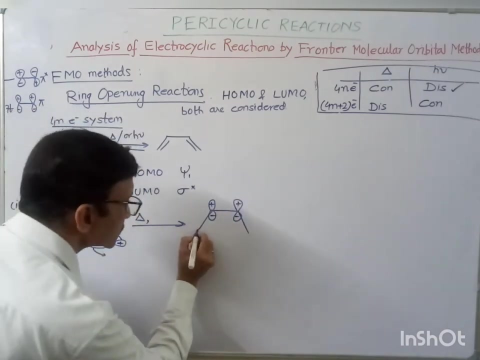 Both orbitals are moving in the same direction. So if this is moving in this direction, then it means this flow will like this, And here this flow will like this, And here this flow will come like this. Okay, So what you will find here. So this is our plus plus minus. 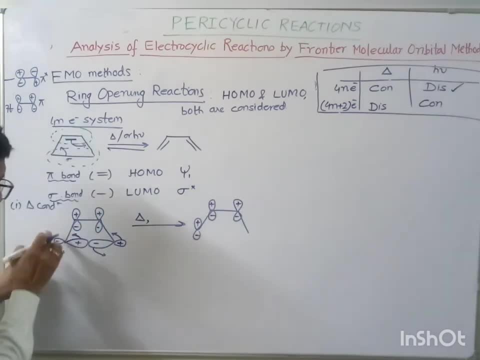 minus, And this is plus. plus is going up, minus is going down. Plus is going up, minus is going down. Plus is going up, minus is going down. Okay, So that is, this is the. this is what I have done here. I have done. now let's see whether this butadiene is formed or. 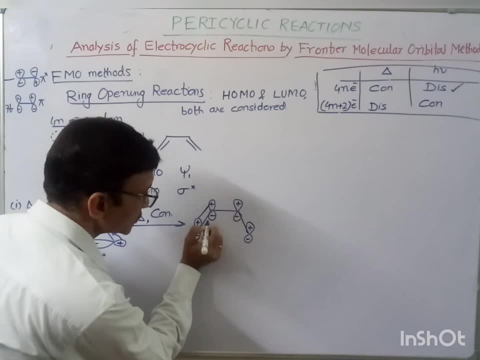 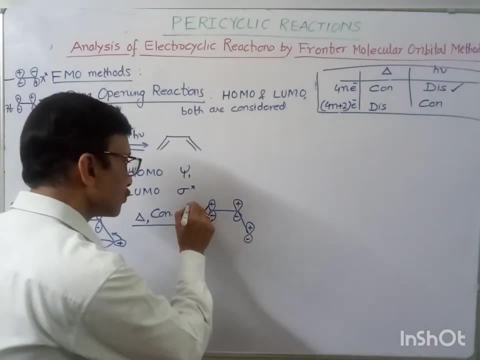 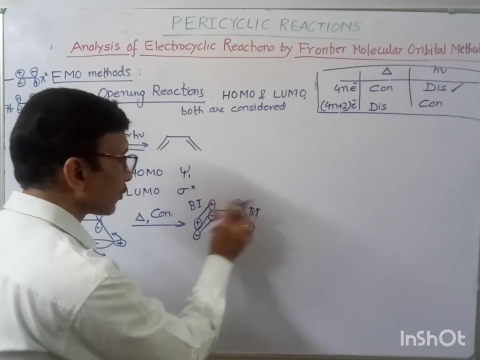 not after opening. so if you will see here this sideways overlap plus plus and this minus minus. this is giving you the bonding infraction and this is also giving you the bonding infraction: plus plus. so bonding infraction, bonding infraction. so this is so either both bonding infraction, 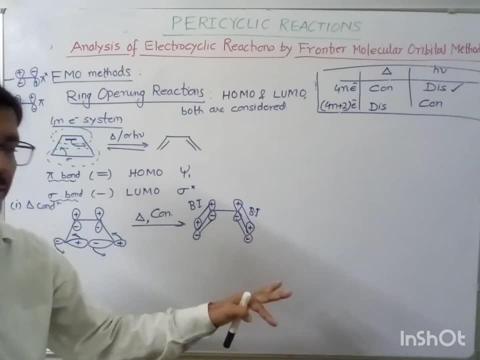 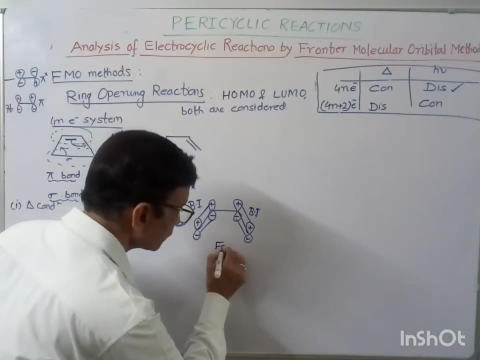 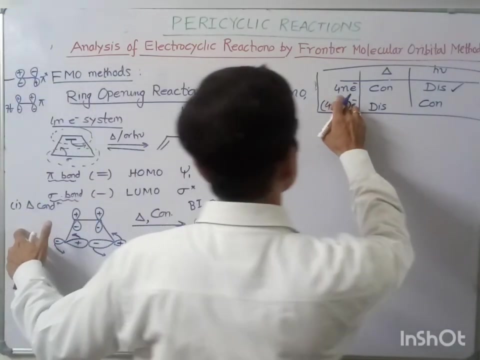 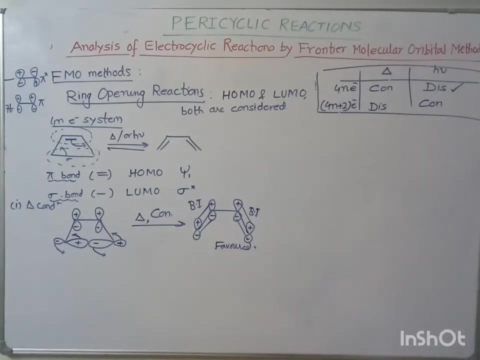 bonding infraction or both antibonding and dividing bonding infraction is favored. one bonding in one anti bonding, that would not be favored. so this is, this is favored. same thing you will see here when for an electron system, for an electron system under thermal condition, the thermal condition, what is going on competition, what is going on on tradition, and if you will see, 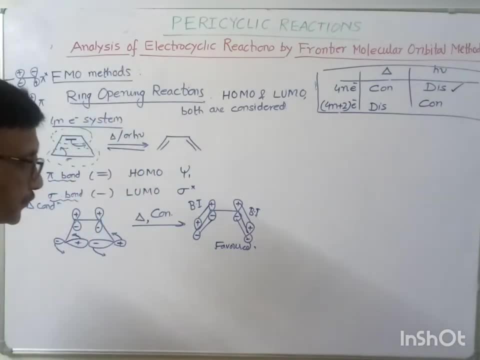 here in pond rotation, what type of? so this is like this. now suppose I do this rotation, then what will happen? if this is moving in this direction, then what you will see? this will move in opposite direction. this should move in opposite direction like this. it is moving in anticlockwise direction. 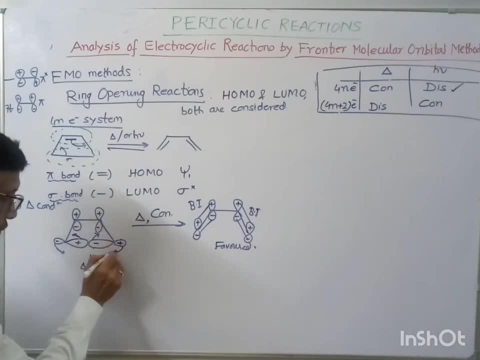 this should move in a clockwise direction. this should move in a clockwise direction like this. so what you will find now you will find: so this is plus, plus, minus, minus. plus is going up and this minus is going up. plus is going up, minus is going down. this 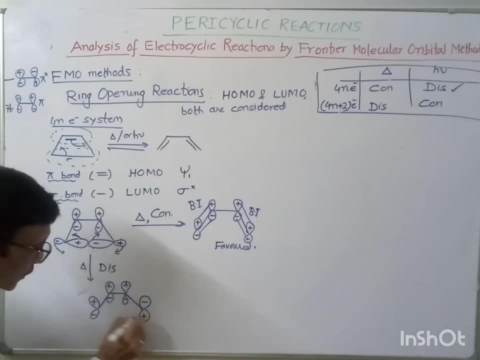 minus is going up, plus is coming down, Like this: what you have seen here, this is bonding interaction: plus plus, and this is plus minus, anti-bonding interaction. this is anti-bonding interaction. is it allowed? 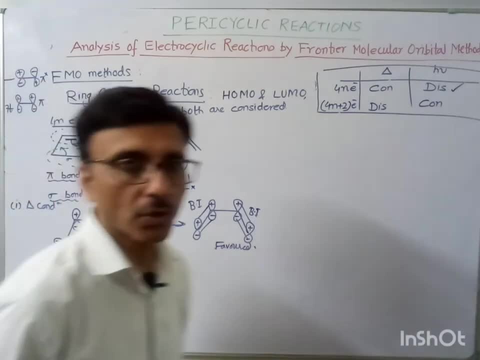 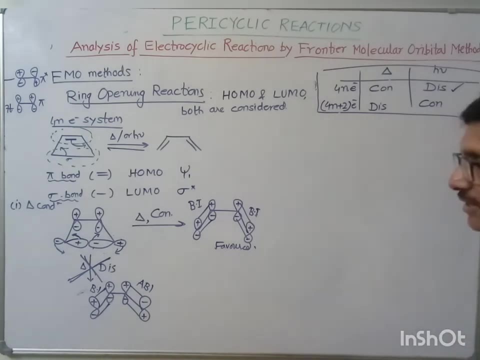 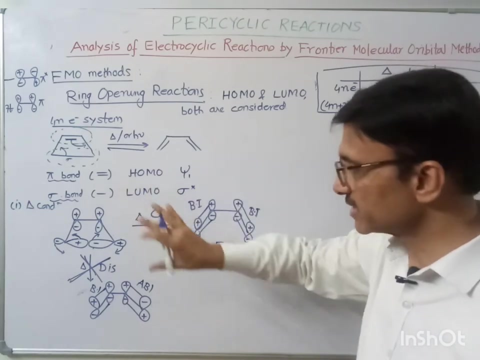 No, this is not allowed. this is not allowed. so like this. so this is the case under thermal condition, so we may also take: this can be taken as a lumbar and this can be taken as a homo also. so the result that would be same result would be same if I take this: 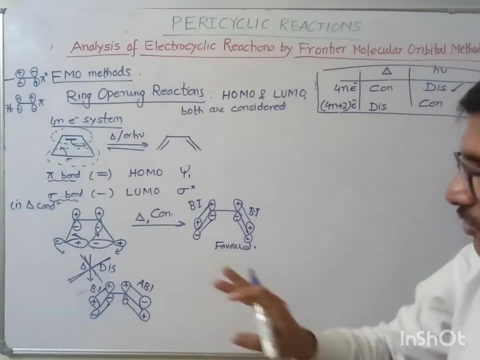 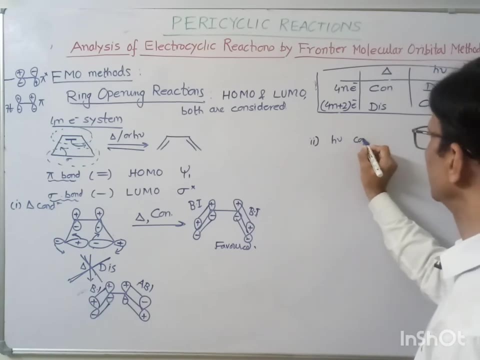 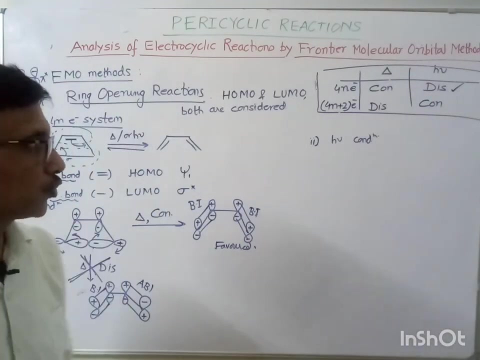 lumbar and this homo then also. result would be same: you can do your stuff. So suppose now, second condition is the photochemical condition. under photochemical condition, let us see. let us see, under photochemical condition, so in photochemical condition. 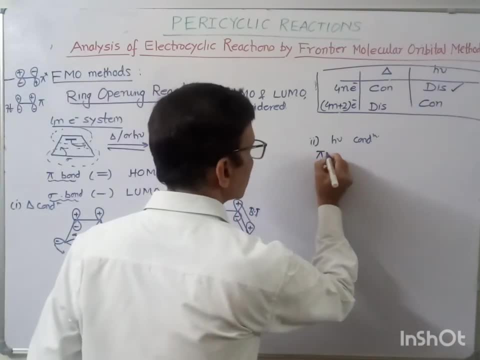 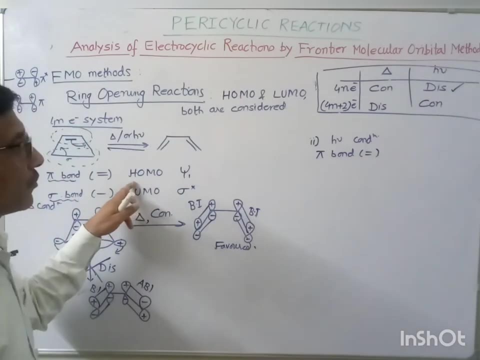 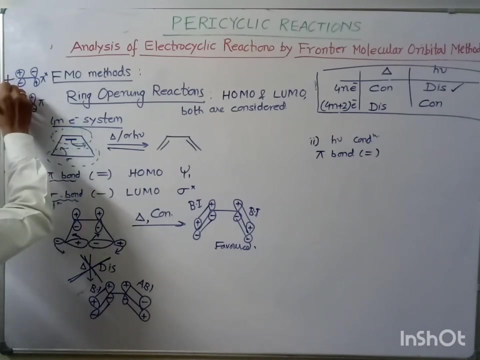 pi bond, suppose this pi bond. So this pi bond or double bond, what should I take? I should take the homo under photochemical condition. so for this homo for photochemical condition, that would be pi star, the one of the left, one that will go over here, and this will now become the homo under photochemical. 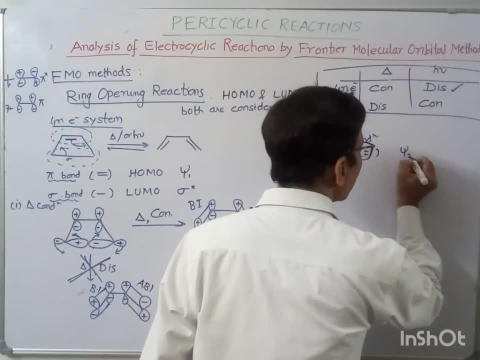 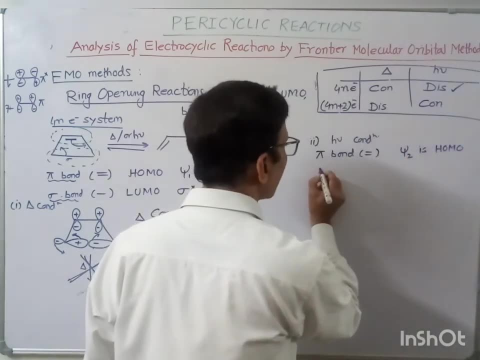 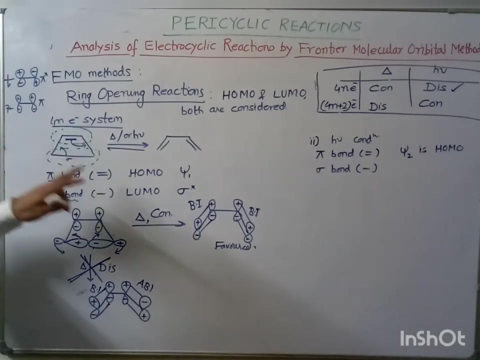 condition. So psi 2,, psi 2 is the homo, psi 2 is, And for sigma bond, that is single bond. what should be the homo? no doubt sigma star, sigma star, and what should be the lumo, here lumo, sigma star would remain as a lumo, so sigma. 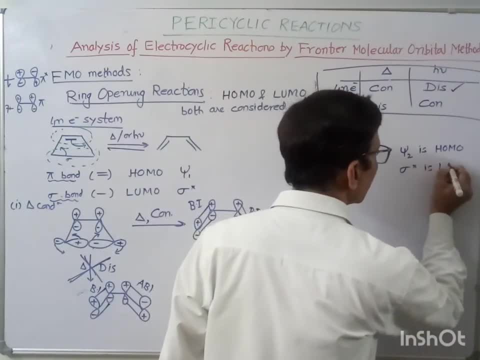 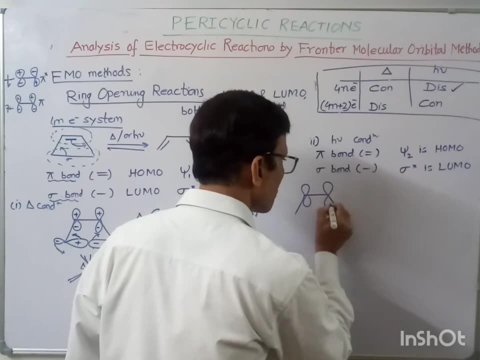 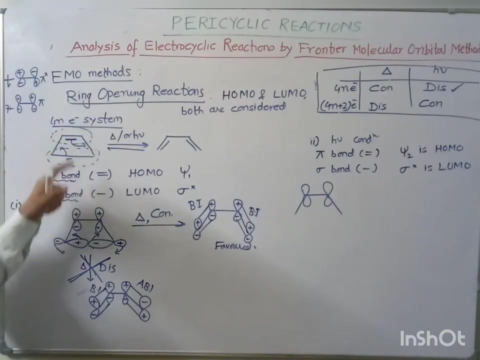 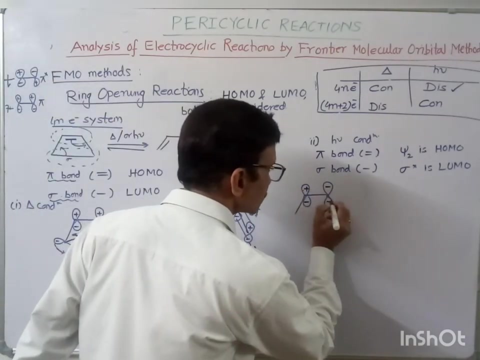 star will remain as a lumo. so now let us see. So this is our homo. homo is psi 2, homo is psi 2, so for ethene system, psi 2, this is all, pi pi star. you can say so, this is plus and this is minus. this is minus now. 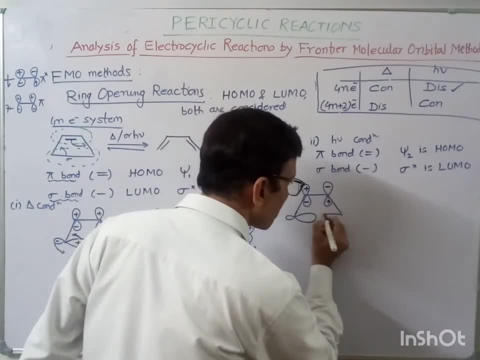 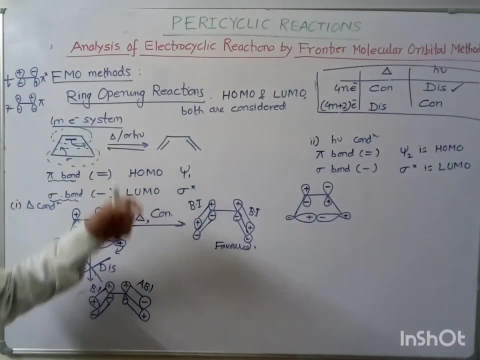 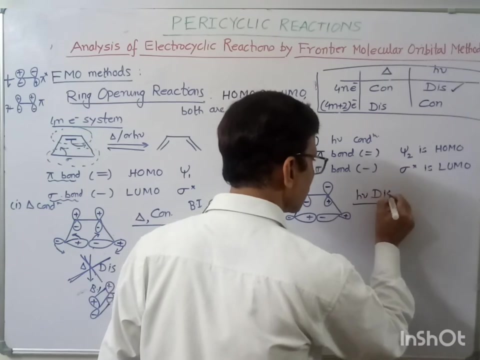 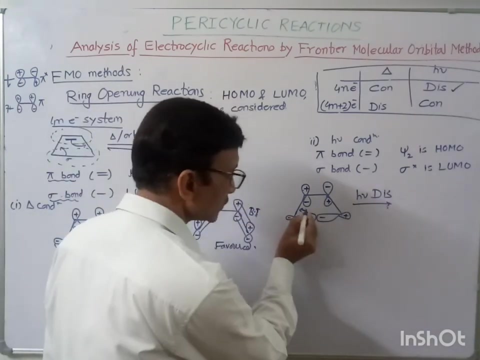 sigma star plus minus, minus plus. so let us open it. open it, if I open it, the photochemical condition, suppose I do the disc rotation, suppose I do disc rotation, then what you will find, you will find, this orbital will move, suppose in a anticlockwise manner, then 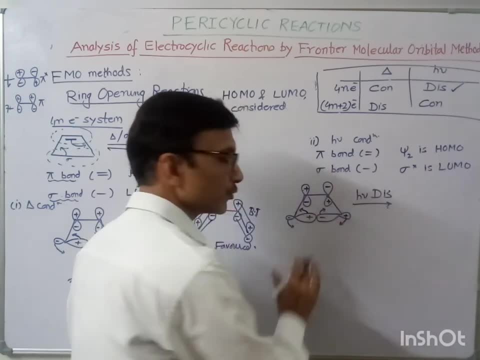 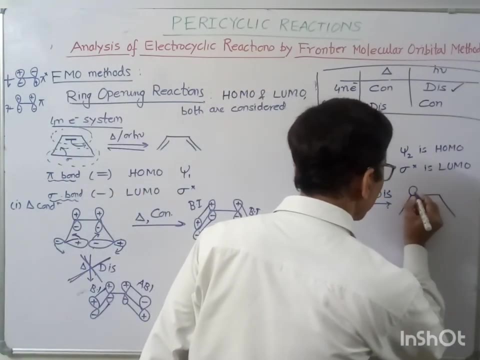 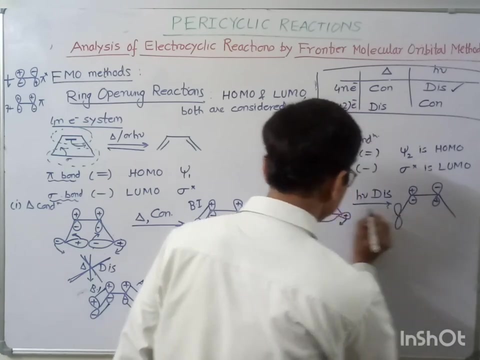 this orbital will move in a clockwise manner means opposite direction. both will open in a opposite direction. so what we can find here? we can find this is plus minus, minus, plus, and this will open like this: So this is going up, this plus is plus loop is going up, this loop is going down in the 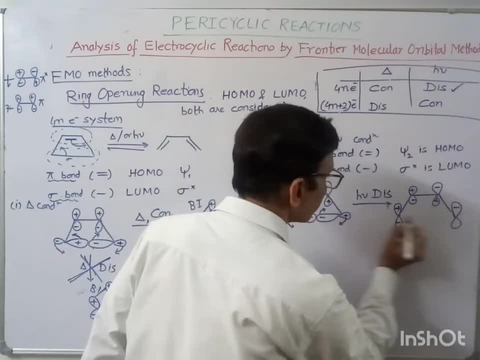 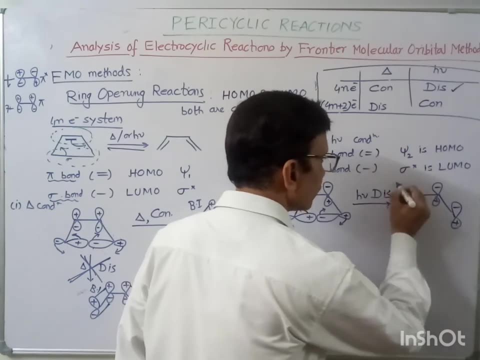 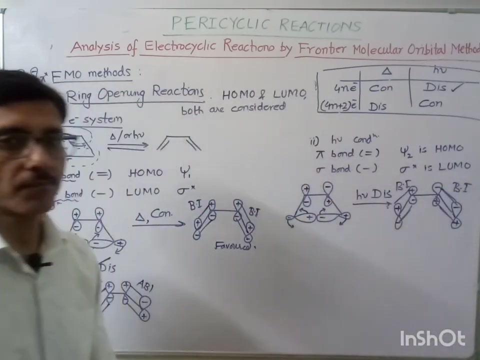 same way, if you will see, minus is going up and plus is going down. so what we have seen- we have seen positive, positive, negative, negative bonding interaction over here and this negative, negative, positive, positive bonding interaction over here. so it means 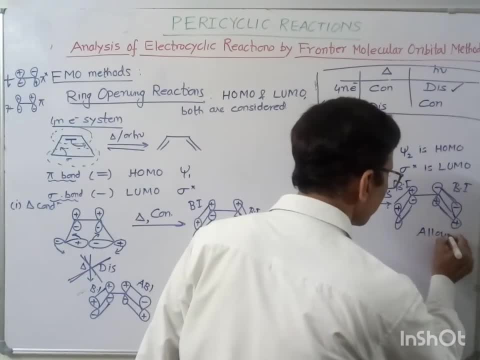 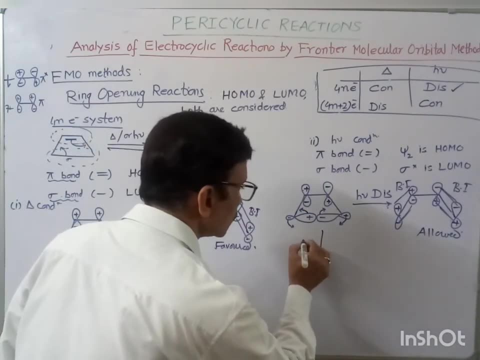 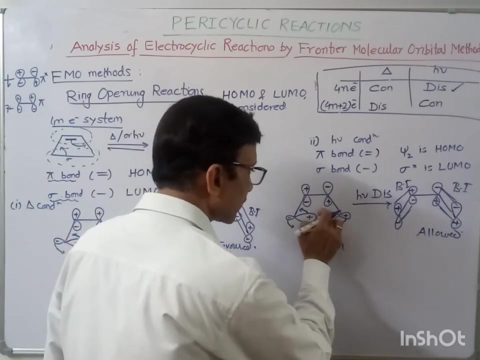 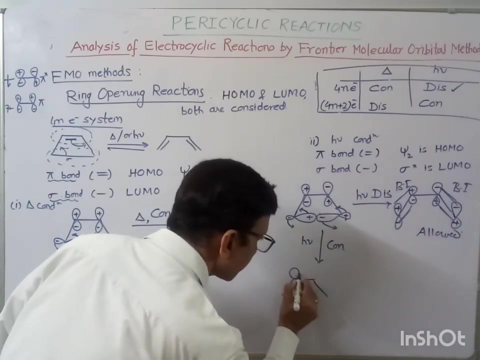 this is allowed. this is allowed over here. Now, if I do suppose, suppose I do under a photochemical condition on rotation, and if this is moving in this direction, then other lobe will also move in a same direction like this. so what you will find here. so this is plus, minus, minus, plus. and now this is: 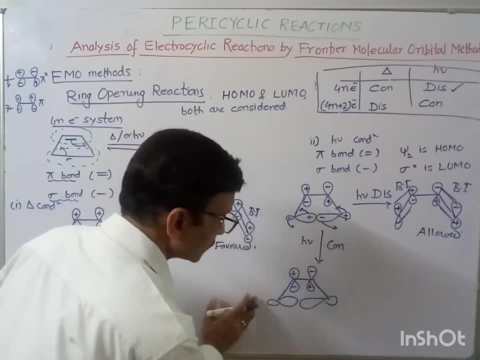 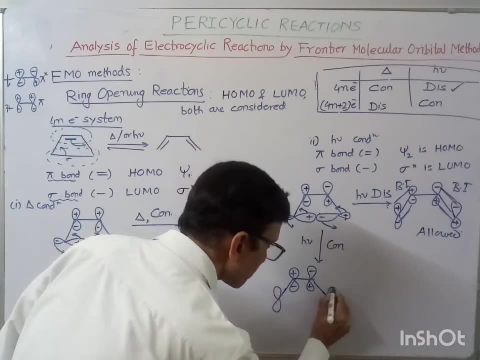 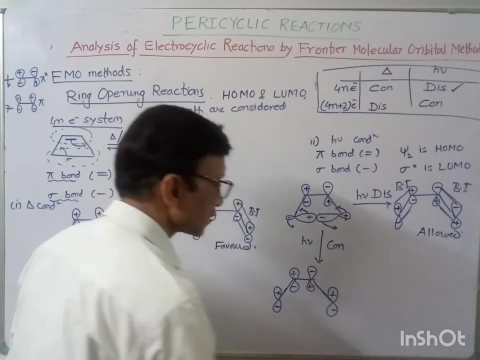 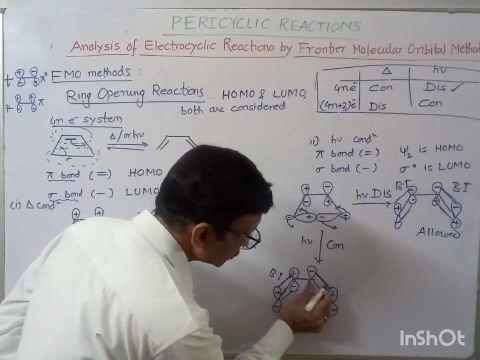 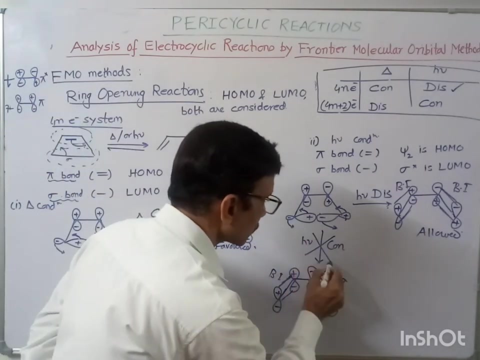 okay. So plus is going up, minus is coming down. plus is going up, minus is coming down. So here positive-positive bonding interaction is taking place over here, but negative-positive, here you will not see the bonding Here, anti-bonding interaction. that's why this is non-positive. 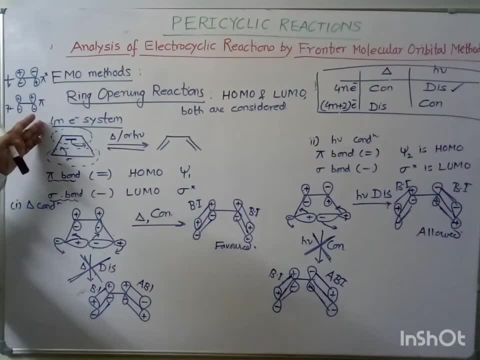 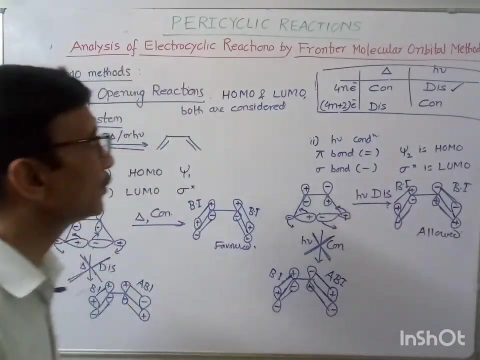 So what we have seen for 4N electron system, for 4N electron system under thermal condition. under thermal condition, con-rotation of this is favored. Under photochemical condition, this rotation is favored. So this we have proved for 4N electron system, 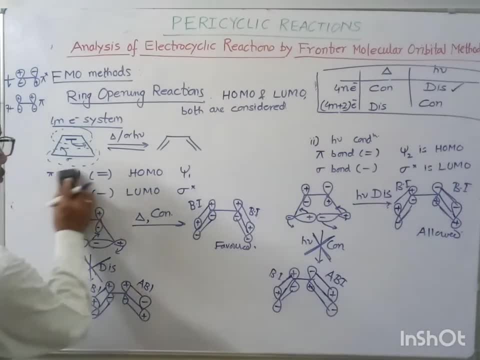 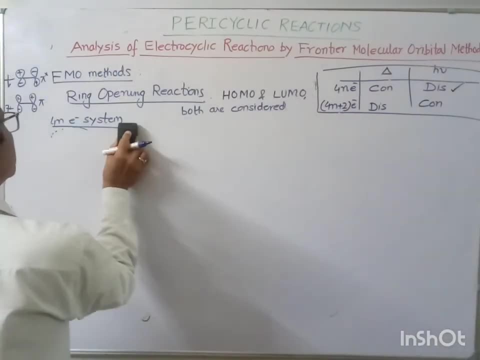 Same thing we can do for 4N plus 2 electron system. So let's see for 4N plus 2 electron system if we will do So here. the feed-through personajes are idling where they are going to. 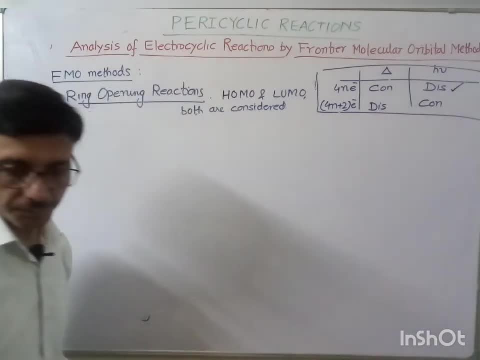 decode the region and then send that check. on this first one, In this case state state with 5N electron, Thank being positive, simple mapping. So the 4N electron was knowledge ofュes they could, I don't know once again, 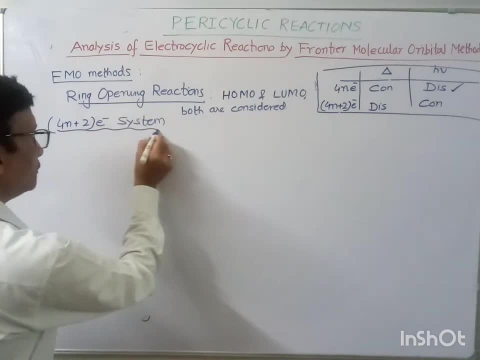 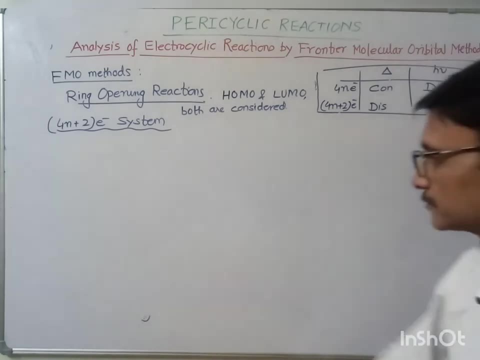 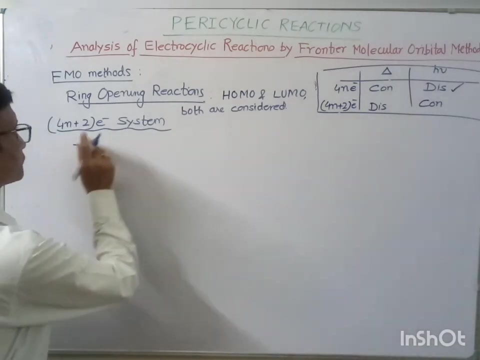 make that soldering a个 4N人民 W. all right, But for 4N electron system, the 4N electron Tambex Now. so let's take the example of foreign plush plushy hand. welche hand? Our hand is not hand hand like this. 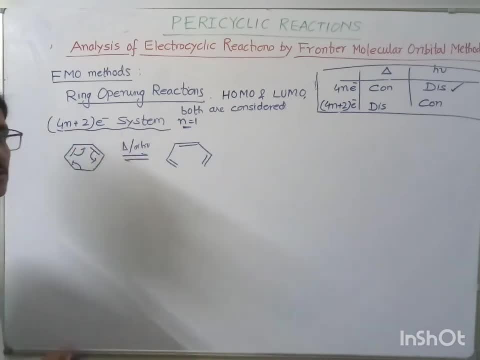 Now you can take it like this: Okay, Okay, Okay, coming out to be 6.. This 6 electron system- this is the example of this- is 4m plus 2 electron system, and this can be analyzed either in the photochemical condition or thermal. 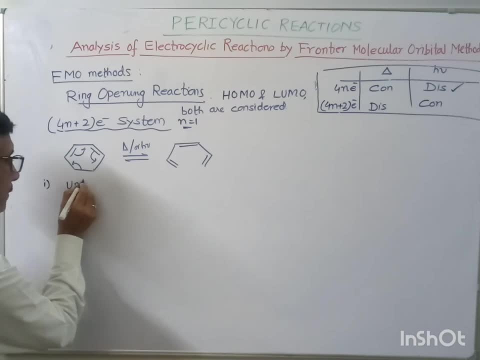 condition. Let us see first under thermal condition, under thermal condition, What we can see over here. under thermal condition, what would be the home of what we have to see, What we have to in this ring opening reaction, what we have to take HOMO as well. 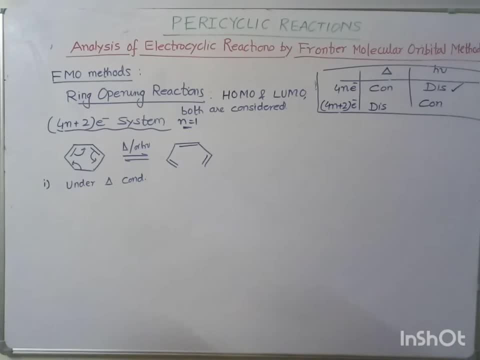 as HOMO. So one of the here, if you will see the reacting partner. again, two reacting partners are there. One of the reacting partner, this is the 9.. Another reacting partner: this is our sigma bond. These are the two reacting partner of the of your reactant. So this: 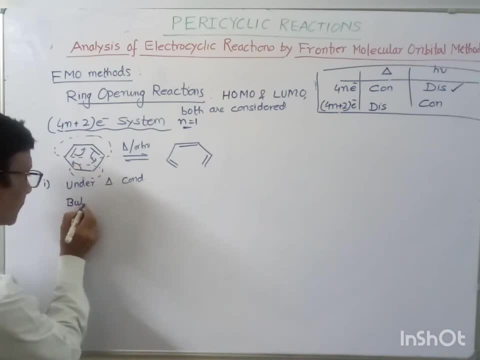 is our sigma bond. First reacting partner is the butadiene. Butadiene is the first reacting partner- Or you can say so- for butadiene. what would be the HOMO for butadiene? HOMO for butadiene is 1,, 2,, 3, 4.. This is butadiene 4 molecular orbital, That is psi 1, psi 2,. 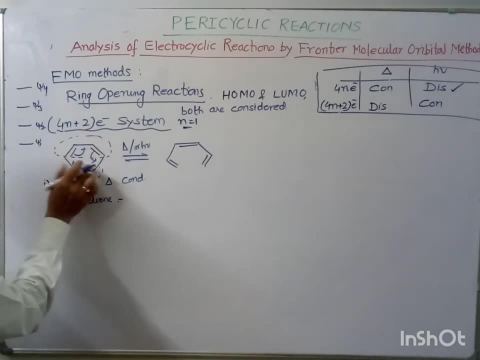 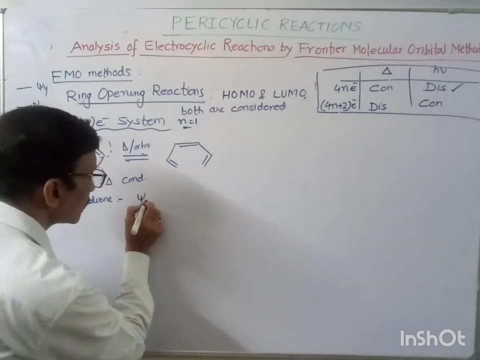 psi 3, psi 4.. So 4 electrons are present in butadiene, So 2 electrons over here, 2 electrons over here. So psi 2 would be the HOMO. Psi 2 is HOMO. Now, this is sigma bond. 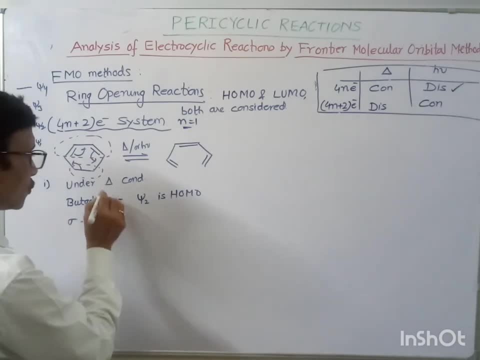 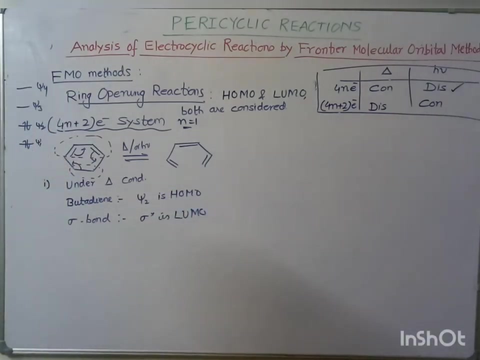 Sigma bond is the another reacting partner. So for sigma bond we have to take the LOMO, Another reacting partner, we should take the LOMO of it. So sigma star is the LOMO. So 1 HOMO and the 1 HOMO and the LOMO that we may take. 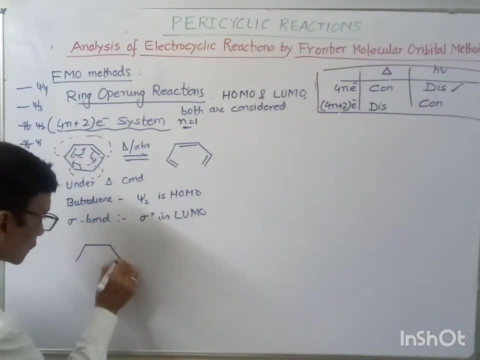 So let us take it. So this is sigma star, plus, minus, minus, minus. Now, HOMO side bond: This end orbital should be end orbital for this butadiene, end orbital for this butadiene. that should be plus minus opposite side. So I am only drawing the end orbital of the 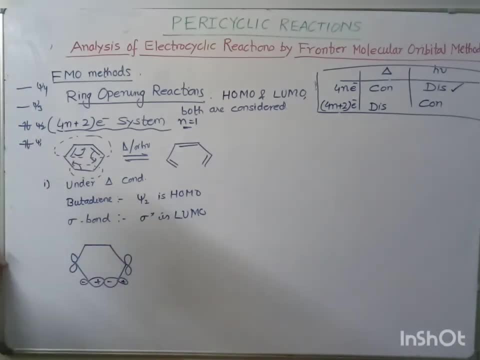 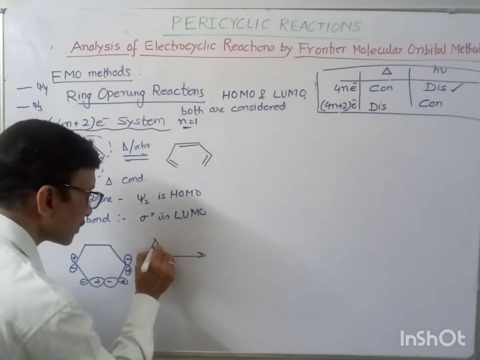 this butadiene. We have to only consider the end orbital butadiene. This is plus and this should be minus. So let's do the ring opening reaction. Suppose I do the on thermal condition, I do this rotation, What I do, This rotation And what you will find here. So this will 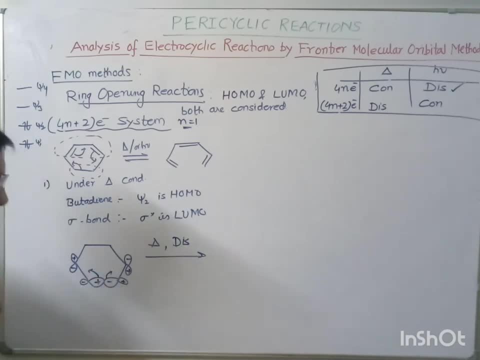 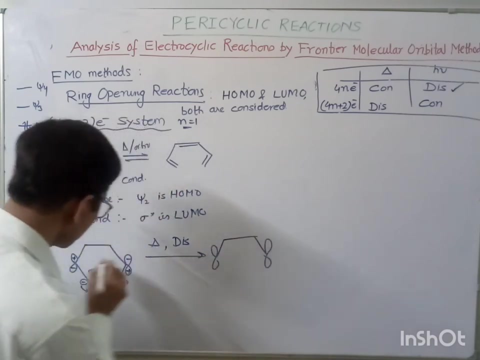 open like this, and this will open in this direction- Opposite direction. So this load will come down. This load will also come down. Minus will come up, What you will see over here. So this is plus, minus, minus, plus. Okay, Plus over. This is plus, minus This. 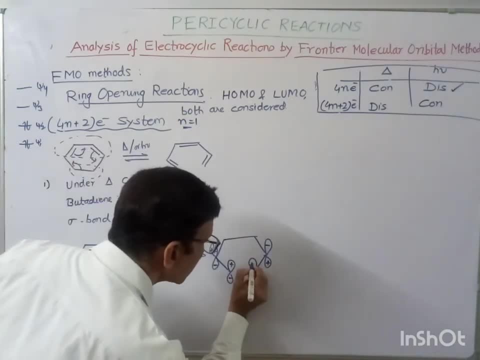 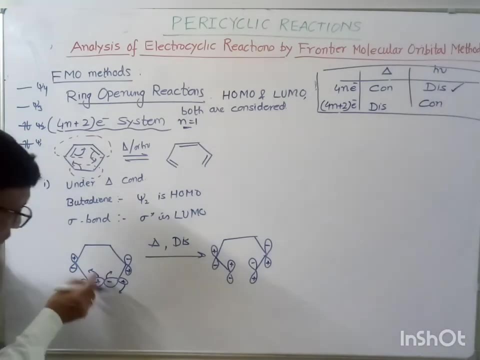 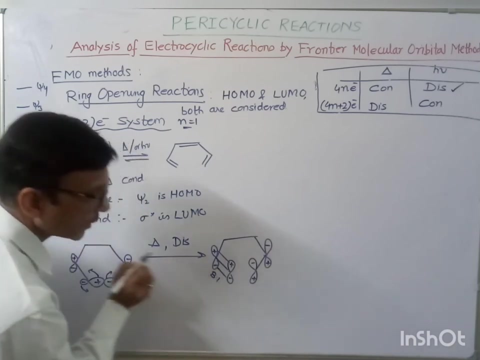 is minus And this is minus, This is plus Okay, This is minus, This is plus Okay. So this is open, This opens. Now a pi bond can be formed like this: This is bonding interaction, And here minus, minus, plus, plus. This is also bonding interaction, So this is allowed. 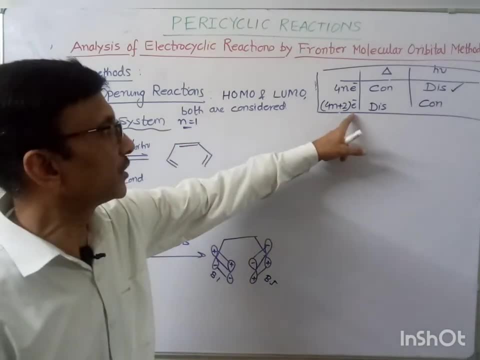 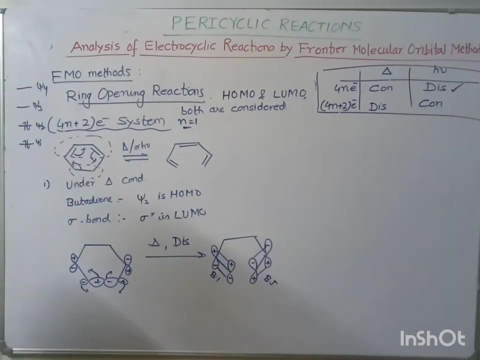 So 4n plus 2 electron system, 4n plus 2 under electron system, under thermal condition, is what kind of rotation of orbital, This rotation, This rotation is allowed. So same thing if you will do under thermal condition Bond rotation, That would be allowed or not. If 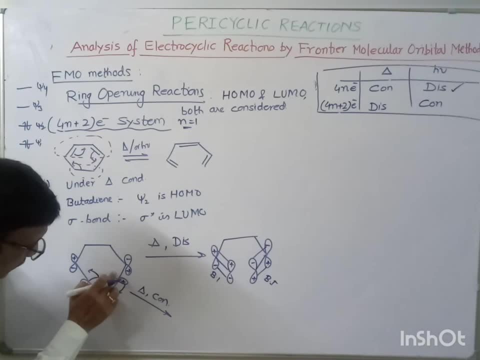 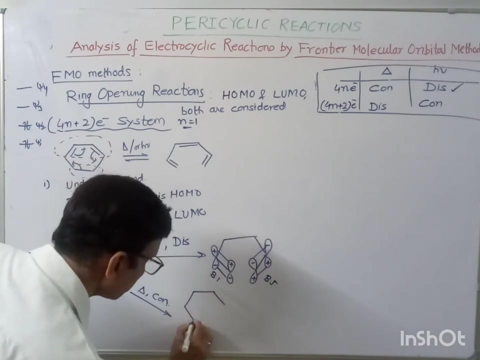 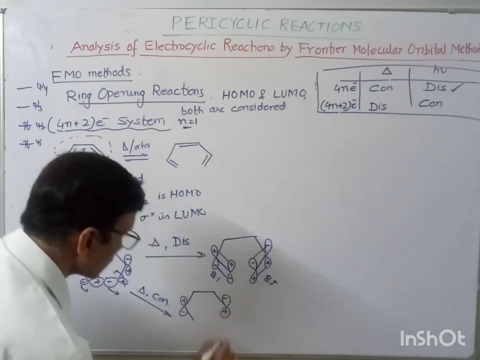 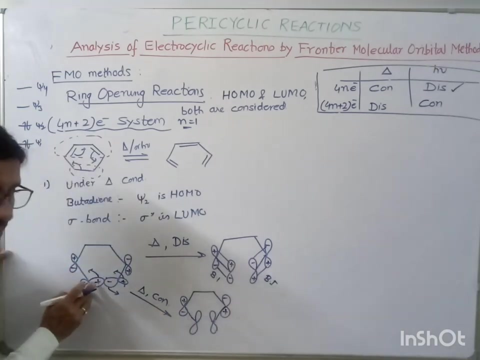 this is moving in a anticlockwise manner, then this should also move in a anticlockwise manner, because in bond rotation both orbital moves in a same direction. This also moves like this, But you will find it over here. Ha, It opens, Okay. So if opens, than So plus sign will go up, Plus Minus sign is going. 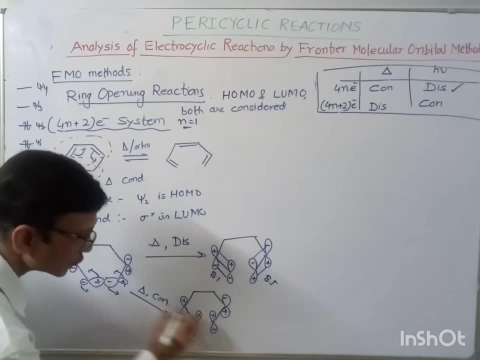 down. Plus sign is going up, Ha, and minus sign is going down. now, if you will see here, this is bonding interaction. okay, but this is anti-bonding. plus minus, plus minus, this is anti-bonding interaction. this is modern. this is on down. so, under thermal condition, what you have seen under thermal condition, this 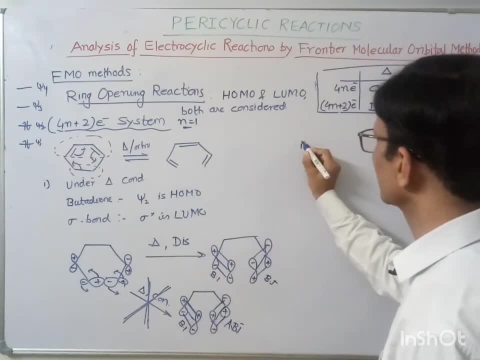 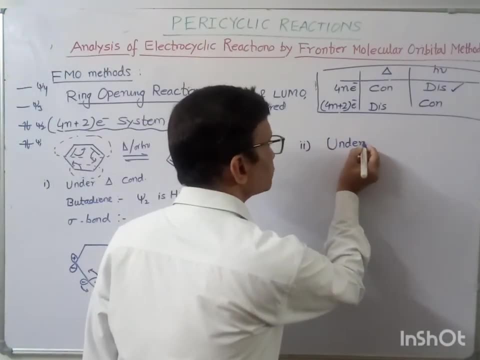 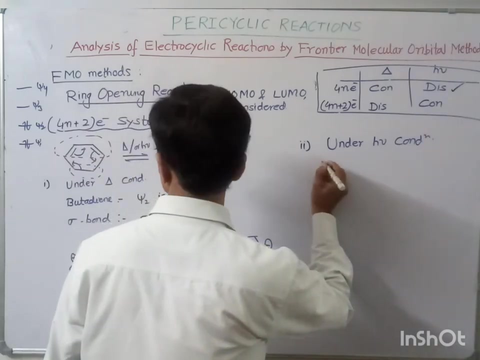 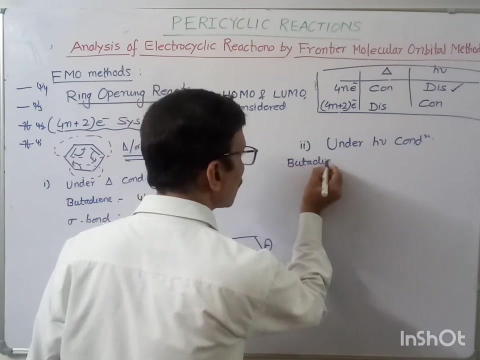 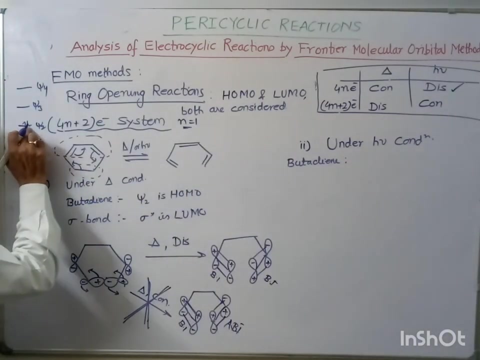 rotation is only allowed. now let's see under photochemical condition. so we will analyze under photochemical condition. okay, so one orbital. so under photochemical condition, if you take butadiene, what would the homo for butadiene, homo for one? under photochemical condition, one of the electron will go over here. 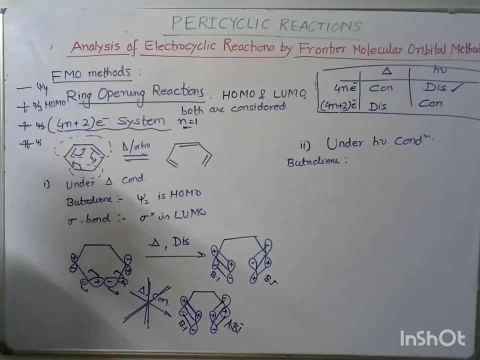 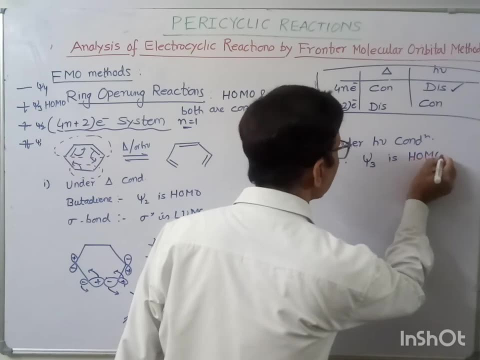 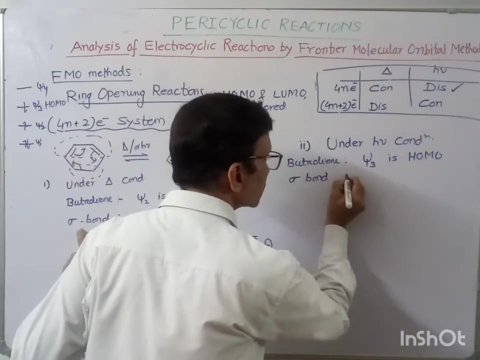 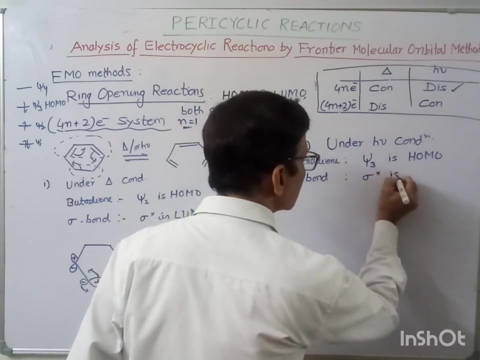 and psi 3 will become the homo here. psi 3 is homo, so psi 3 is homo and lumo for sigma bond. for sigma bond is another reacting partner for sigma bond. the lumo that would be sigma star will remain as a lumo. okay now. 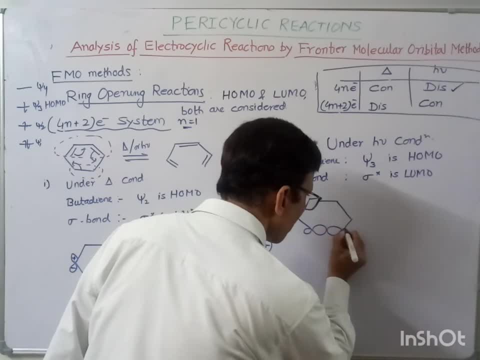 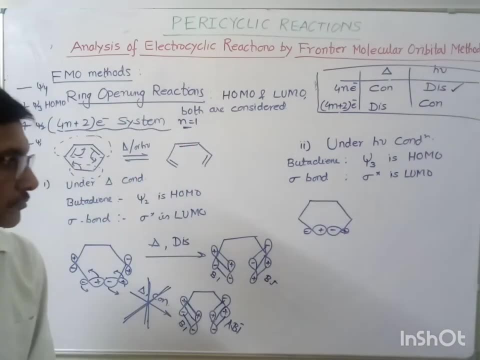 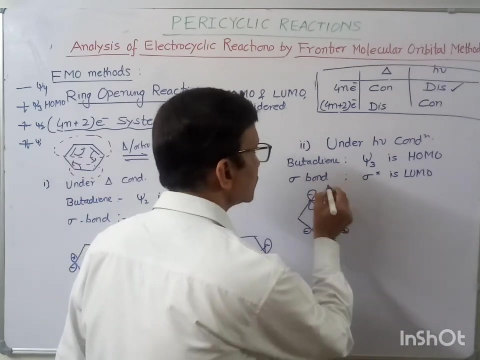 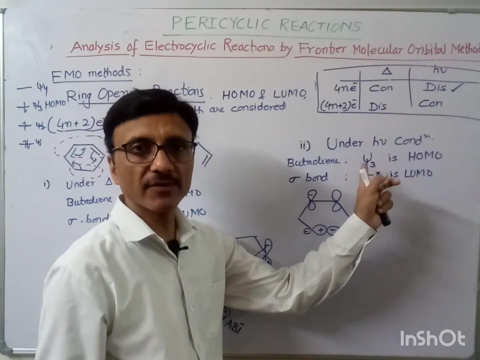 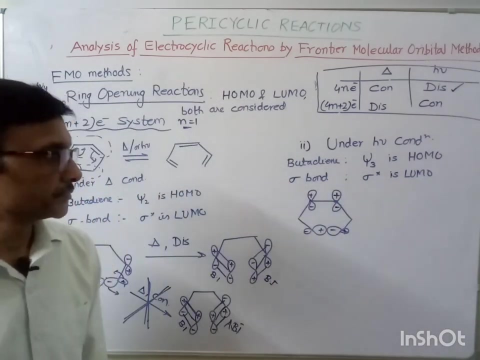 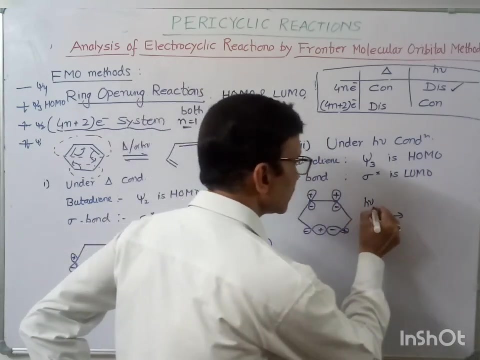 for sigma bond will remain as a lumo right for처�. частly nonelse breaks, and so it depends on the. this is how it looks like, so we will manage server Now. let's open it under photochemical condition. under photochemical condition, let's do the. 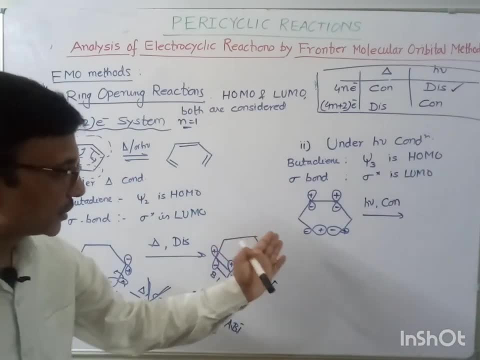 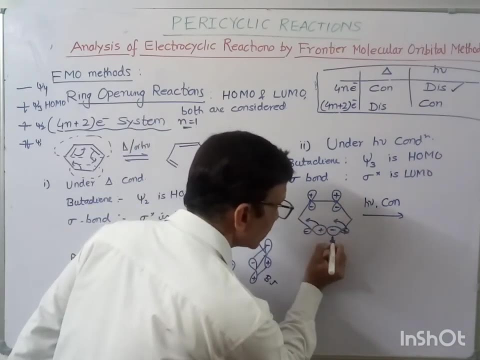 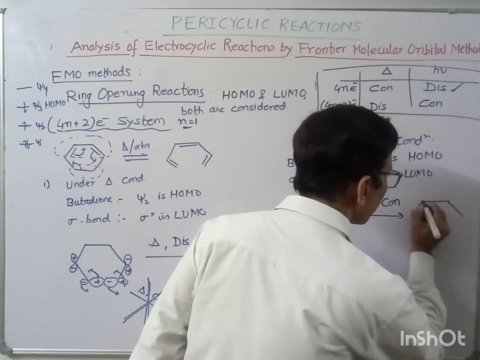 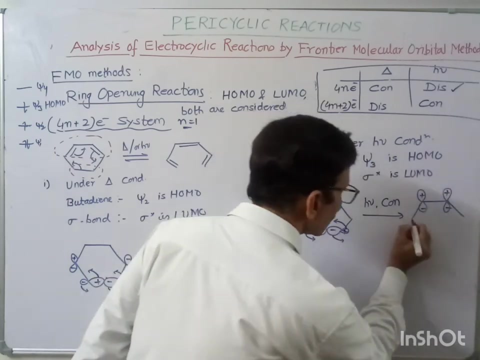 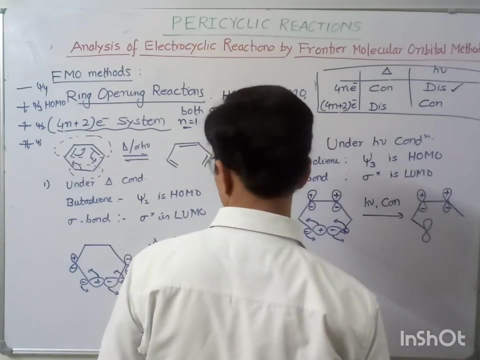 corn rotation. Corn rotation means this orbital opens in the same direction. if this is opens like this, then this will go over here, this will go down and this will go down What you will find. so plus plus, minus, minus. so this opens. sorry, so I have to. 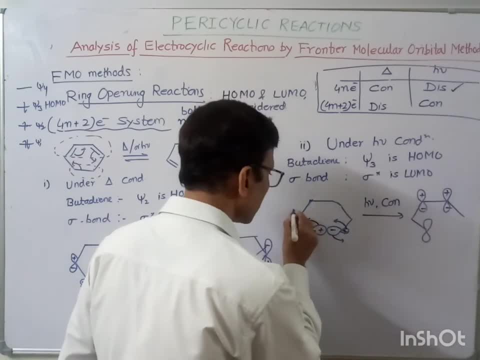 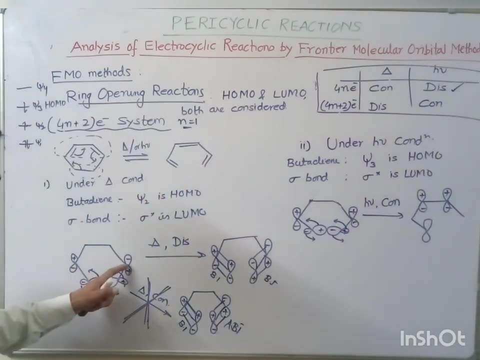 write for butadiene, so for butadiene the low will come over here: plus plus, minus, minus. Ok, So with low for butadiene, end lobes are present over this corner, so end lobes are. 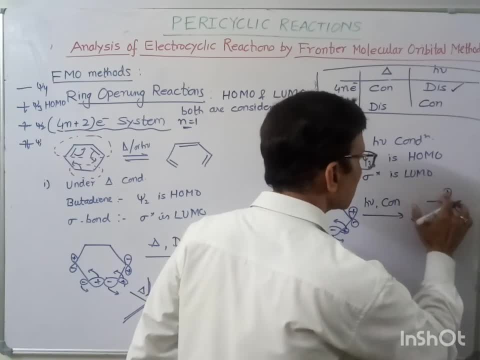 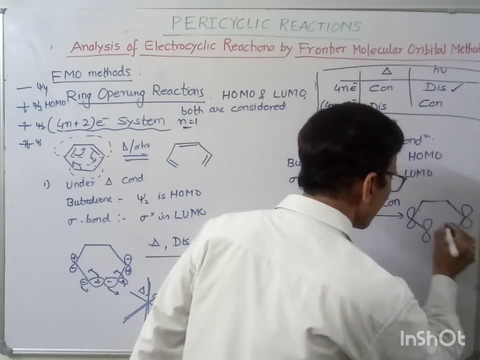 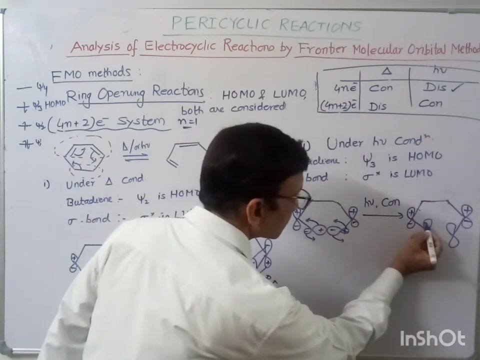 present over this corner, so I should correct it. ok, so no doubt this will have the plus, plus, minus, minus Now. so if you see this, plus will come up, minus is coming down, plus is coming up, minus. 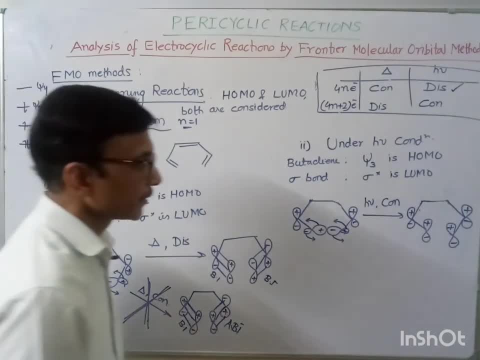 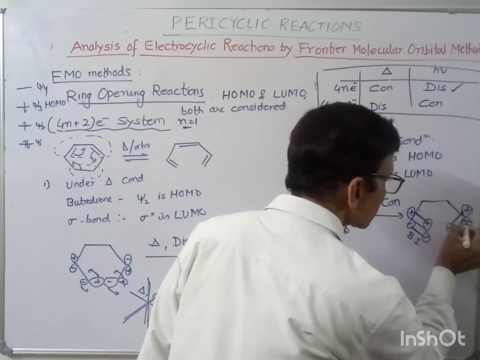 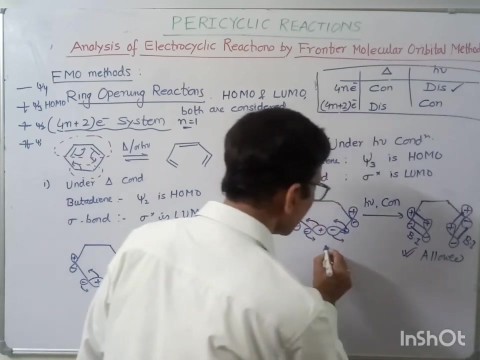 is coming down like this: ok, So, whether bonding interaction plus plus, minus, minus, yes, bonding interaction here also plus plus, minus, minus. bonding interaction, it means, this is allowed, this is allowed. and if you will do the this rotation, if you will do the this rotation, it means, if this: